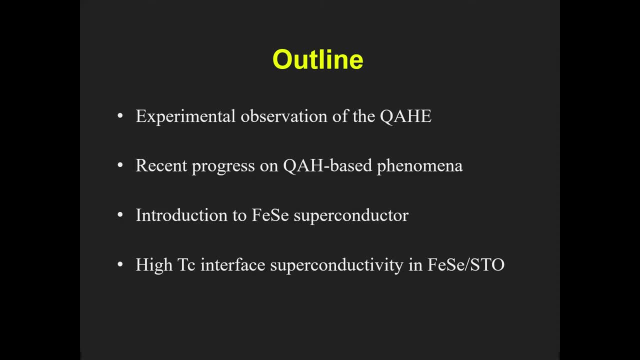 So here's the outline. In the first part I'm going to first show you the experimental observation of the quantum anomalous Hall effect. Basically it's a prelude for, somehow, to Professor Kang Wang's talk. Then I'll show you some variations. progress on quantum anomalous Hall-based phenomena. 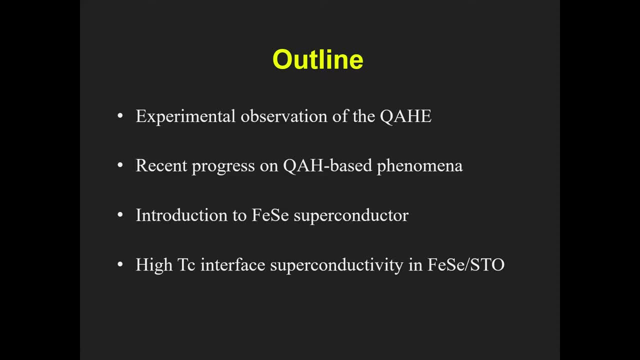 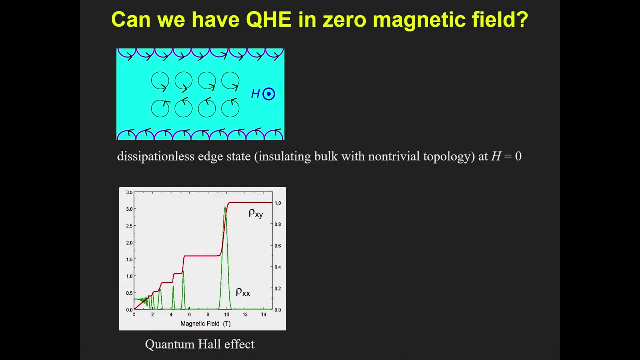 Then in the second part I will show you the interface: high-temperature superconductivity of a monolayer of ion selenide on STO substrate. So here's the original. on motivation. It's an old question, As Duncan mentioned. the question is: can we have quantum Hall effect in zero-magnetic field? 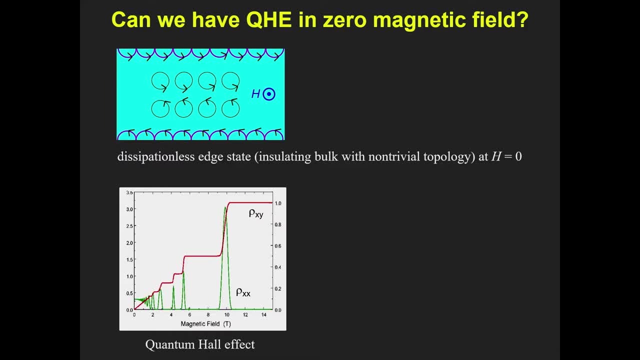 This is the picture for the quantum Hall effect in high-magnetic field, where the magnetic field creates discrete columnar level. localize the bulk state and have this dissipationless chiral edge state which gives you the quantum Hall conductance. Then in zero-magnetic field, it seems too good to be true. 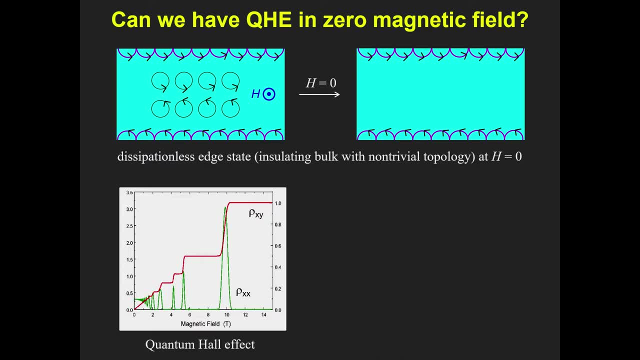 Even without magnetic field, somehow the bulk is still insulating as there's still chiral edge state propagating along the sample edge. From the experimental point of view it means even in zero-magnetic field there's a finite Hall resistance and it's quantized. 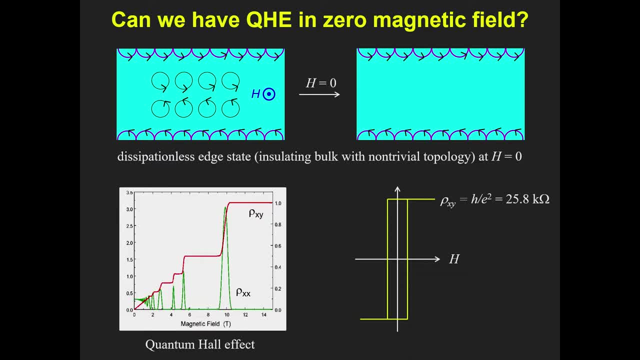 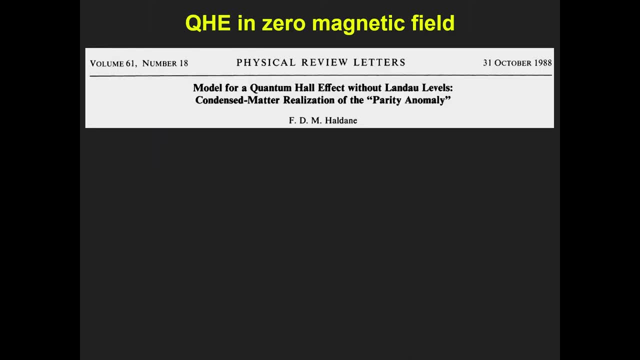 It's around 21.8 kiloohm. You know this loop is called an anomalous Hall effect. This quantized version is called a quantum anomalous Hall effect. This is a further theory about that by Duncan in 1988.. 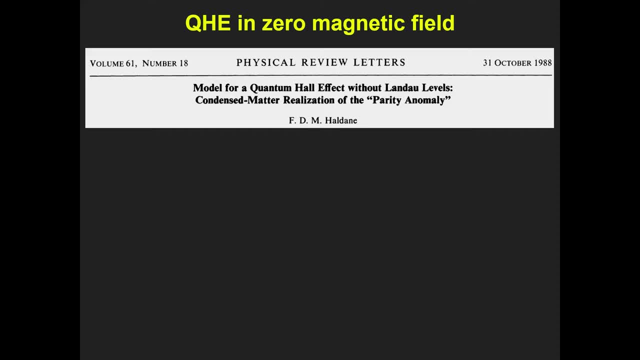 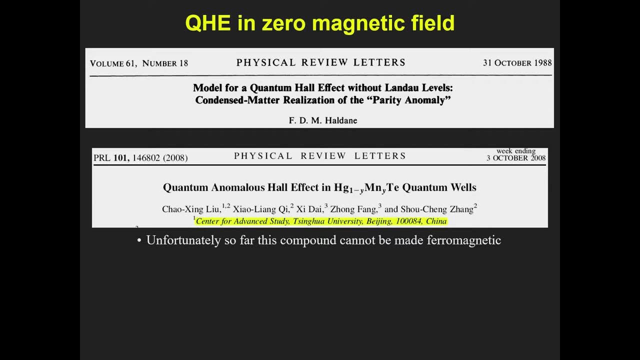 But as he said it's a toy model, He never imagined it could be realized experimentally. Twenty years later, Chao-Hsing Liu and Shou-Cheng Zhang proposed that in mercury telluride- this was at that time- was recently discovered by Professor Molkamp's group to be a 2D topological insulator. 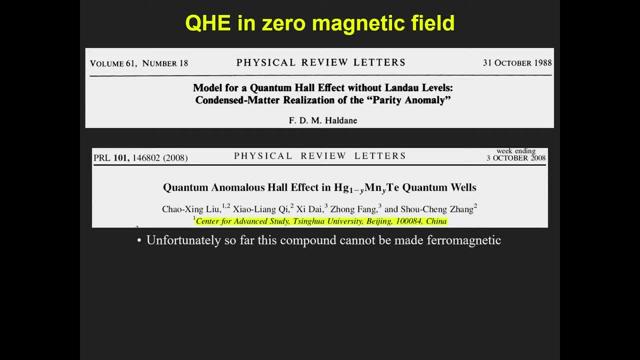 or quantum spin Hall insulator. Chao-Hsing proposed that if you can make this material ferromagnetic, it could be a good material system for realizing quantum anomalous Hall effect. At that time, Chao-Hsing was still a student in our department. 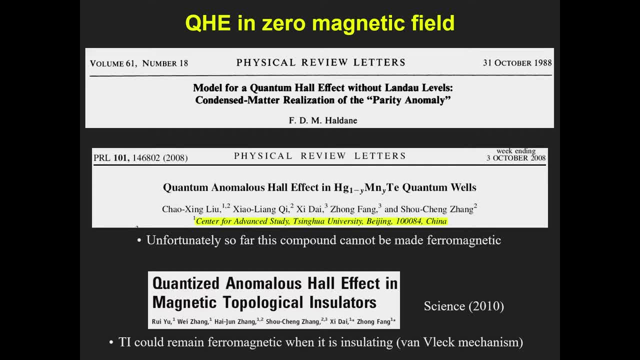 And two years later, Zhong Fang and the Sides group from IOP in Beijing proposed that the 3D topological insulator bismuth selenide, bismuth telluride and antimonyl telluride 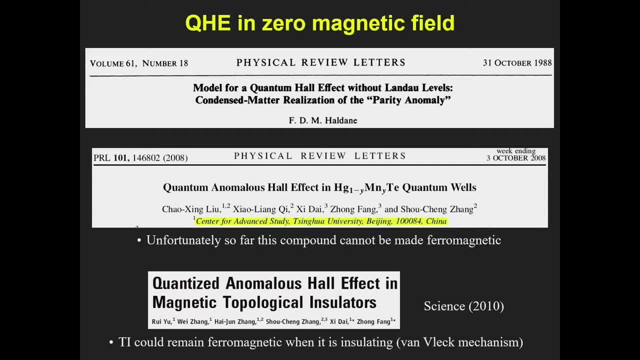 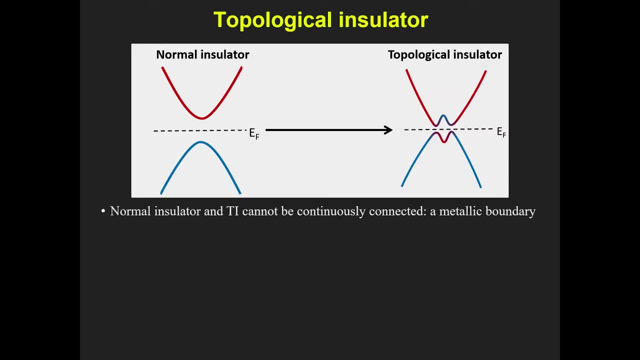 could be an even better system for quantum anomalous Hall effect, because this material can become ferromagnetic even when it is insulating. I think that's a problem for this system. Somehow it still cannot be a spontaneously ferromagnetic. yet This material they proposed are topological insulators. 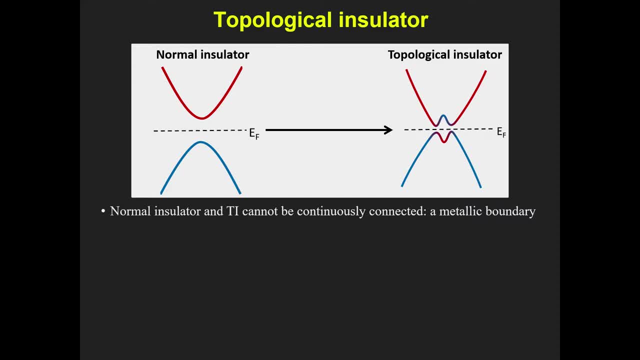 So there's a very simple diagram showing what is a topological insulator And it's consequence in quantum anomalous Hall effect. So this is a band structure of a normal insulator And this is a topological insulator with inverted band structure. 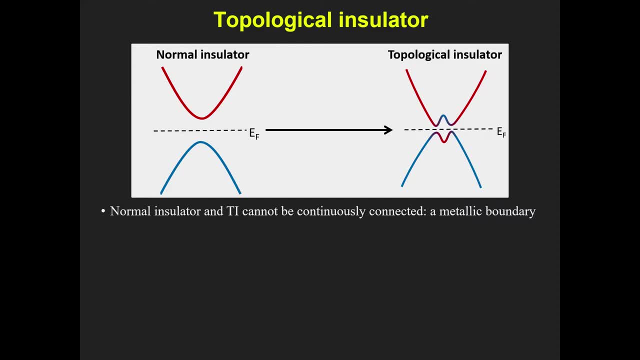 Because they belong to different topological classes and the boundary between them. the gap must close. So there's a topological protected metallic boundary state For 2D topological insulator. it means there will be helical edge state around the sample edge. 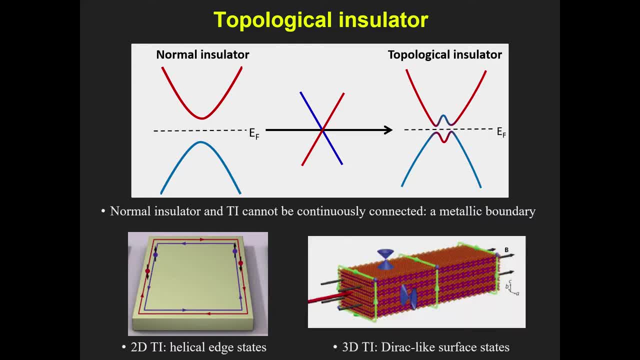 where you can see the quantum spin Hall effect And for 3D topological insulators, there will be this Dirac-like surface state surrounding the whole sample In order to realize the quantum anomalous Hall effect in a topological insulator. 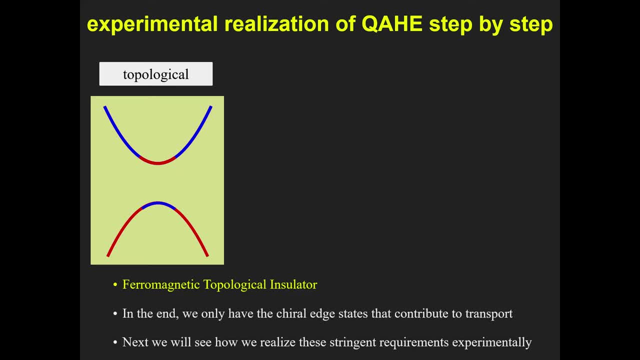 there are three requirements that has to be met simultaneously. First, the sample has to be topological, So there will be surface state or edge state without strong magnetic field. Secondly, the sample has to be ferromagnetic, so that you will have anomalous Hall effect. 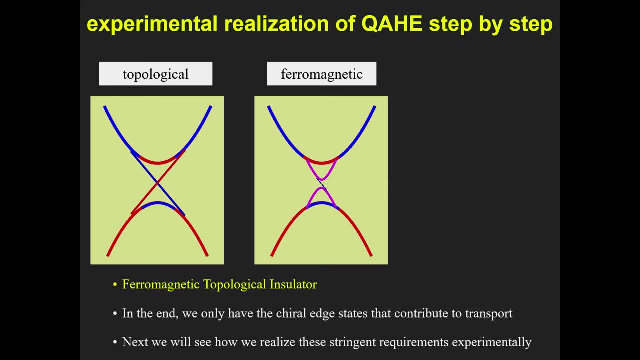 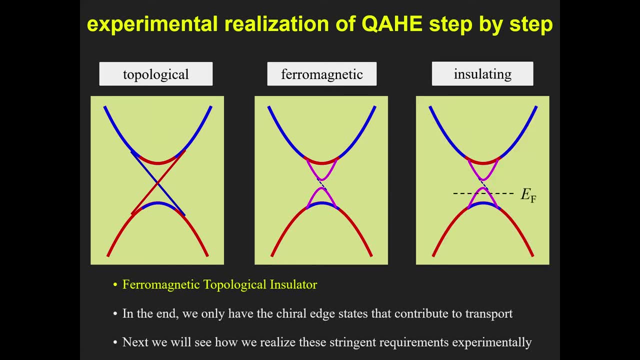 even in zero magnetic field, And also the ferromagnetic order will open a gap at the Dirac point of surface state, So only the edge state will be left. Thirdly, the material has to be truly insulating. That means you have to tune the Fermi level very accurately. 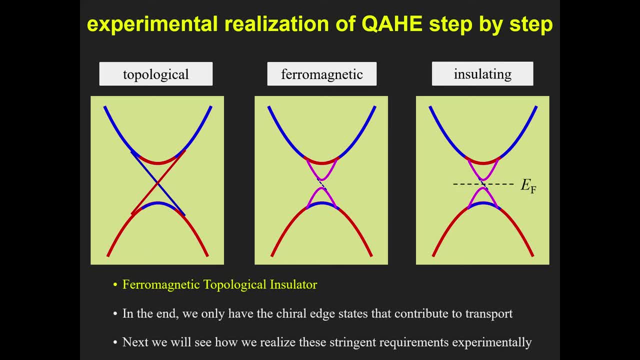 into the energy gap on all the other states And in the end, only chiral edge state will contribute to transport. So what we are looking for is a ferromagnetic topological insulator, And it's not easy to get that because we know that most insulating materials 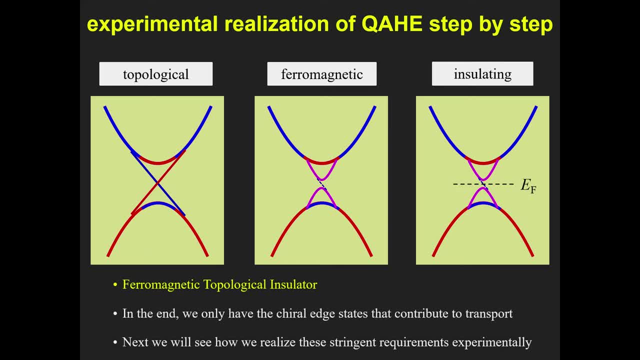 are not ferromagnetic. Very few of them are. Secondly, if the ferromagnetic order is very strong, it can also destroy the topological band structure. So to have these all three parameter conditions met in one material is very difficult, And we will show you how we realize this step by step. 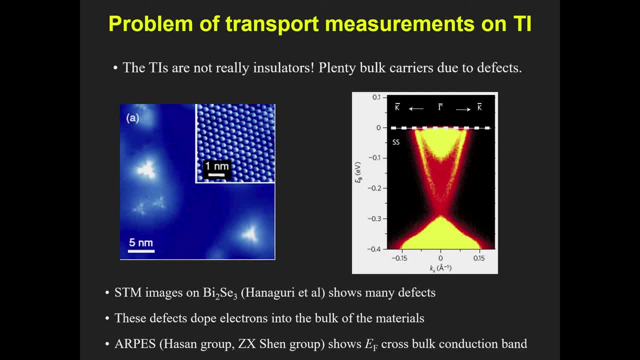 Of course, we encounter a lot of different problems. To show you just one simple problem, that is, all these topological insulating materials that we mentioned: bismuth selenide, bismuth telluride. they are not truly insulating. 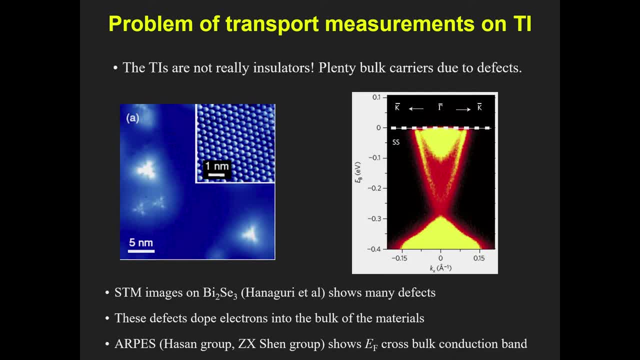 They are actually pretty metallic. This is because when the materials are grown there are always defects in the material in the bulk And most of the defects don't need to charge. So that when you measure the band structure using RPAS by, say, Dakhis Hassan's group. 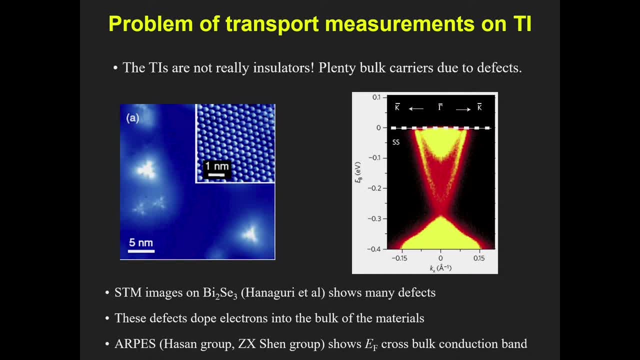 or Ziak-Shen's group. you can see the Fermi level actually cross a bulk conduction band in bismuth selenide and bismuth telluride. That's because the tellurium and selenium vacancies will donate electrons into the sample. 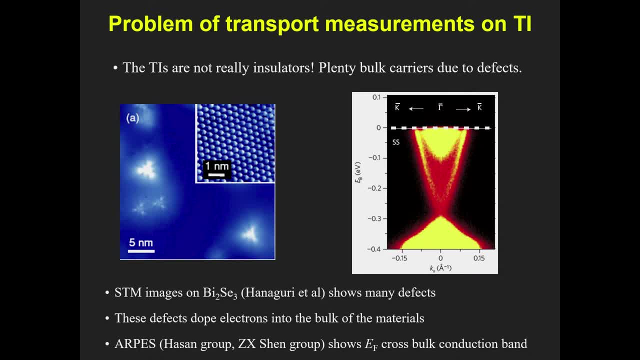 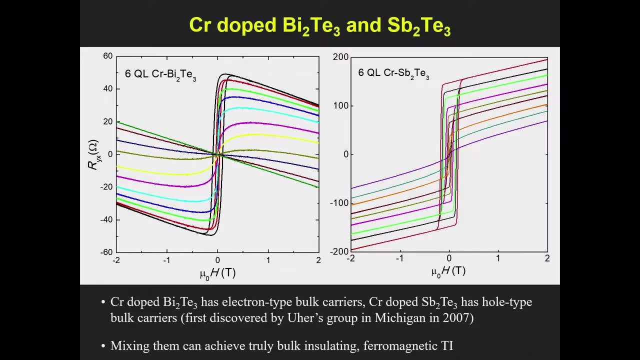 so the bulk is highly conductive. In that case you cannot distinguish bulk surface and agitator transport. This is why, when we try to make this material magnetic and measure the quantum anomalous Hall effect, we found that although this material is truly ferromagnetic, 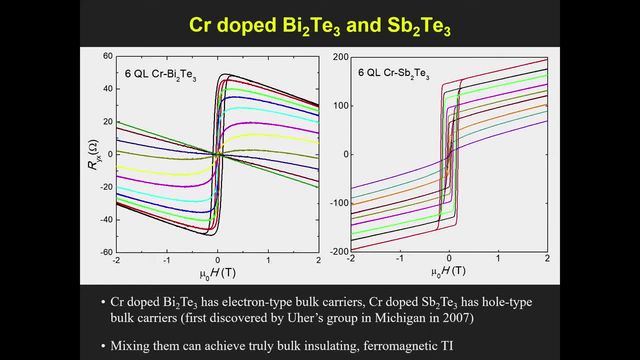 but anomalous. Hall resistance at zero magnetic fields is very tiny. For example, in chromium, the bismuth telluride, it's only about 50 Ohm, and for chromium-doped animal telluride it's only a little more than 100 Ohm. 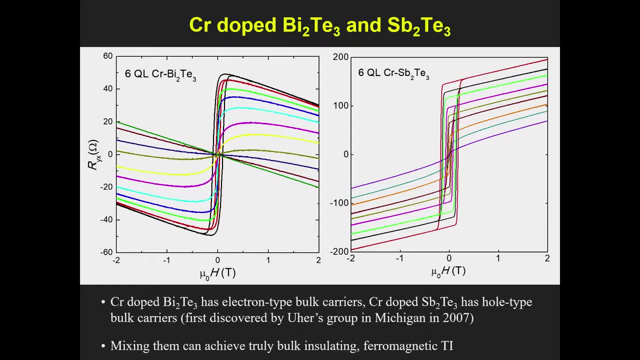 It's far, several orders of magnitude smaller than quantum resistance. This is because you have a lot of bulk carriers in the material. But when we stare at this sample, this data, long enough, we realize in this material the ordinary Hall effect has a negative slope. 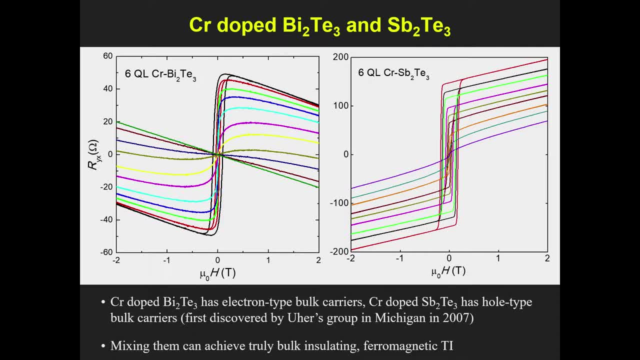 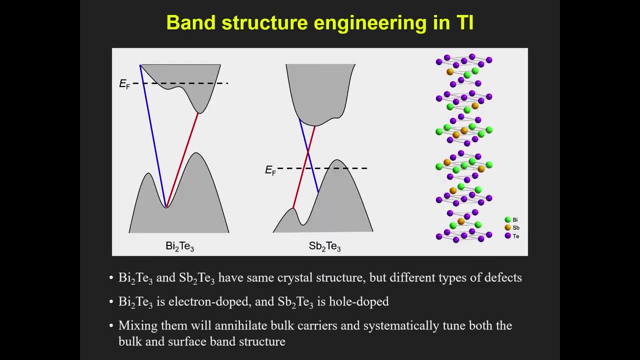 meaning there are electron-type carriers. But for this material- chromium-doped animal telluride- it has a positive slope, meaning there are Hall-like carriers. Then we look at the band structure carefully. This is the band structure of bismuth telluride. 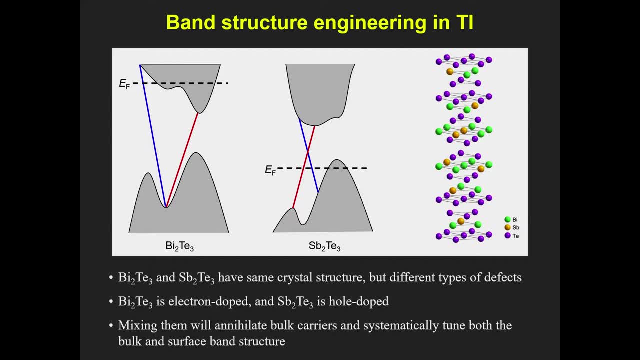 The Fermi level usually lies in the conduction band because the vacancy of tellurium will introduce electrons, But for antimony telluride, the typical type of defect, the anti-side defect which donates Halls. So the Fermi level lies in the valence band. 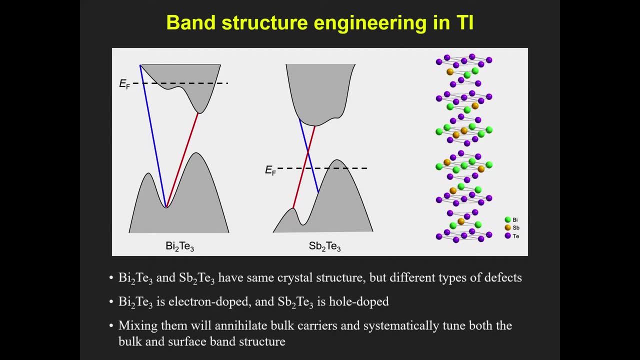 So we thought by mixing these two materials, because they are very similar chemically, we may actually tune the position of the Fermi level very accurately And at some point, if we are lucky enough, we will have a truly insulating material with the Fermi level less close to the direct point. 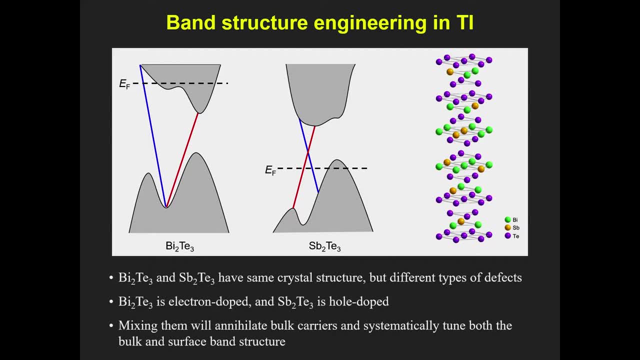 This idea is actually very similar to in the 3-5 semiconductors in gallium arsenide, aluminum arsenide. By mixing them we can tune the energy gap almost continuously. So similarly we have this band structure engineering technique in topological insulator. 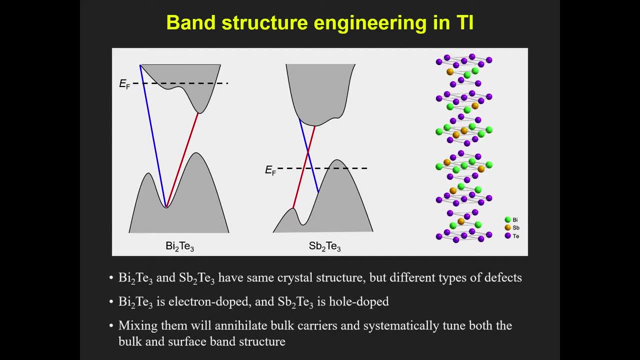 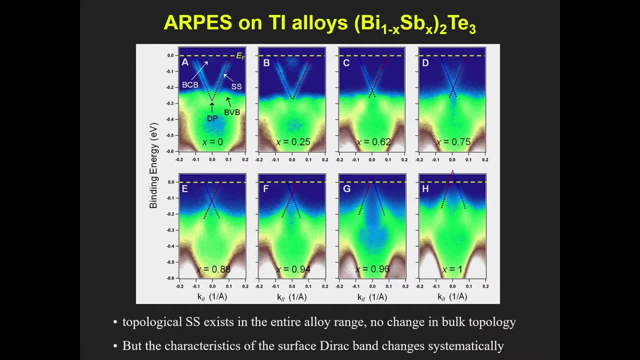 where we can tune both the band structure and the position of the Fermi level. So we draw theories on materials from bismuth telluride over here to antimony telluride and perform r-pass measurement. So, starting from here, the Fermi level really. 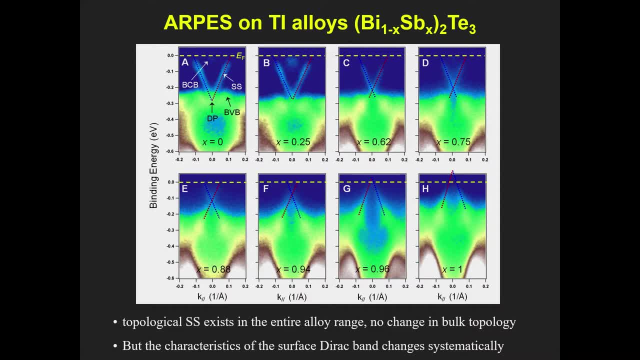 cuts through the bulk conduction band. But as we add antimony into it, you will see the Fermi level moves down continuously towards the valence band and in pure antimony telluride indeed, the Fermi level is very close to the bulk valence band. 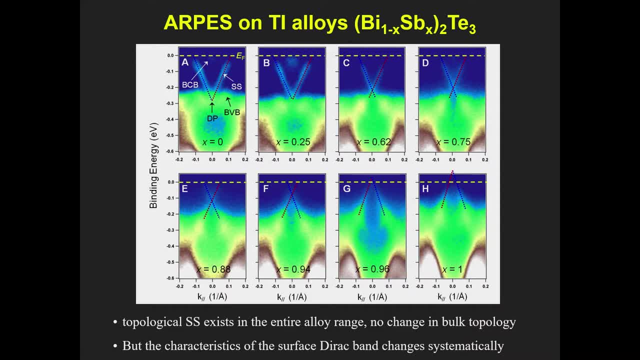 In this regime, with antimony content around 0.94 and 0.96, there's a change of electron type dr cone to a hole type dr cone. So in this area the bulk is truly insulating and we can tune the carrier type. 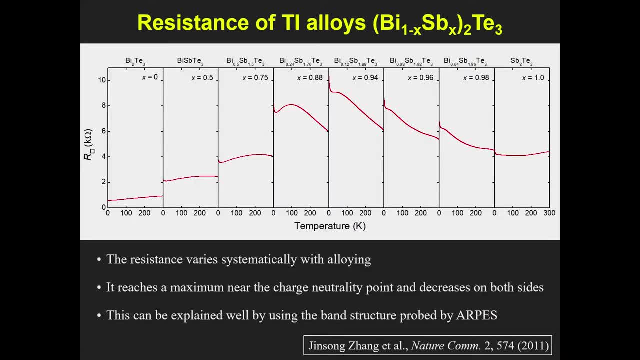 by a bismuth and antimony ratio. We perform transport measurement in this series of ternary alloys and you can see in the two ends pure bismuth telluride and antimony telluride. they are pretty metallic But in the middle somewhere around 0.94,. 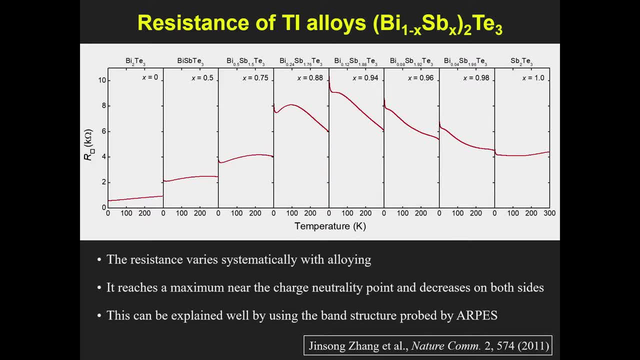 the material is truly insulating. So over here we already have a topological insulator. So two conditions are fulfilled. Then what about ferromagnetic order? Then we try to dope with chromium. Actually we tried several different kinds of doping. 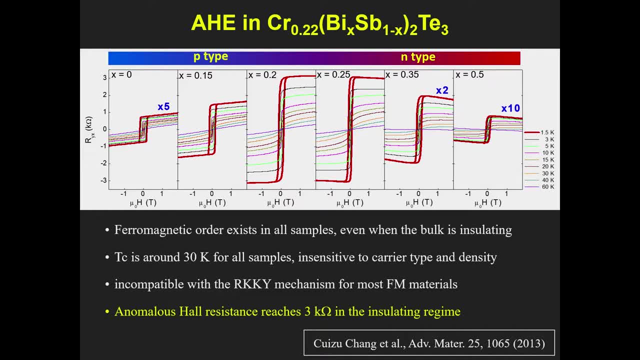 Turns out, chromium works the best When we dope chromium into this alloy. luckily we can see ferromagnetic order across the full phase diagram, not only in pure phase bismuth telluride and antimony telluride, but also in this insulating regime. 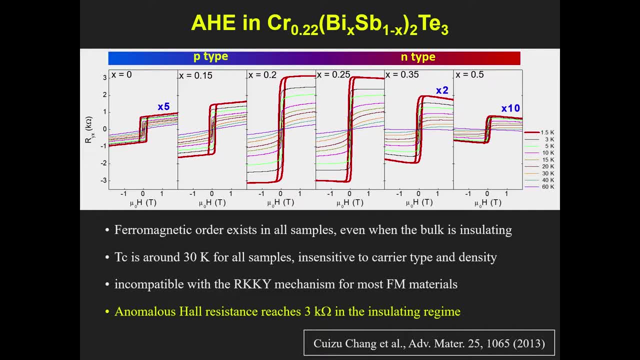 You can see, here we have a hole type carrier, p-type carrier, Here we have n-type carrier In the middle. that's an insulating regime, but the ferromagnetic order is still very strong, The Tc of all these materials. 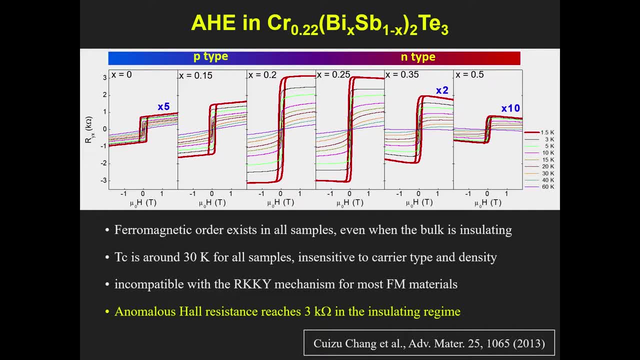 are around 30 Kelvin. It's totally insensitive to carrier type and density. This is very surprising because most ferromagnetic material, the mechanism for ferromagnetic order, is Rkky mediated by attuner carriers. It's very sensitive to carrier type and density. 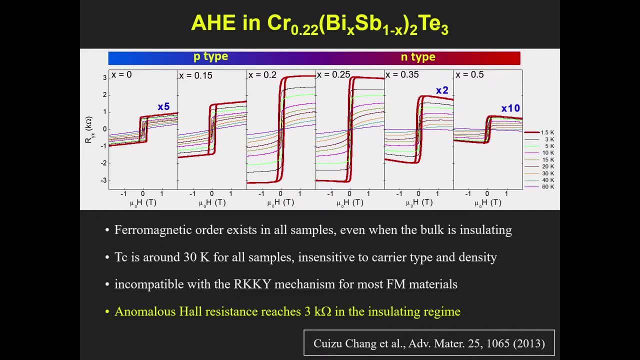 But in this material, as proposed by Feng Zhuang and Dai Xi, it's due to the FLEC mechanism, which is from the band structure, now the attuner carrier. It's not sensitive to attuner electrons and it could be ferromagnetic in the insulating regime. 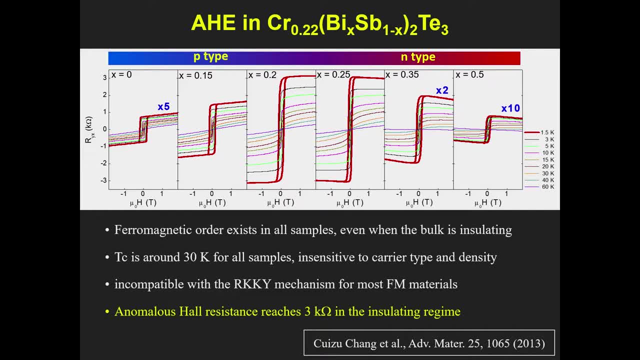 Up to here, we already have a ferromagnetic topological insulator and we know we are very close to the quantum anomalous Hall effect. But that's not enough. You can see now the anomalous Hall resistance is about 3 kiloohm. 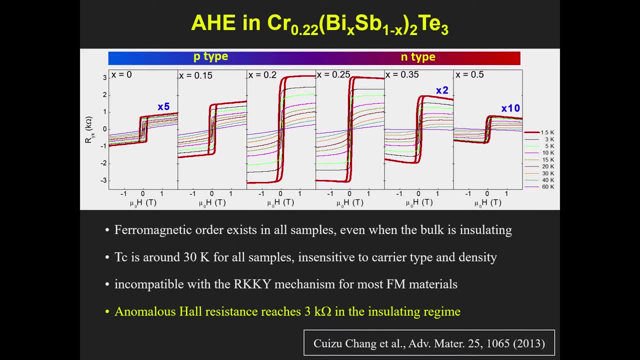 It's still order of magnitude from the quantized value. The reason is, when we grow this material by chemical doping, you can only get a discrete doping level and the chemical potential is not very accurately controlled. In order to achieve that, we have to add a gate voltage. 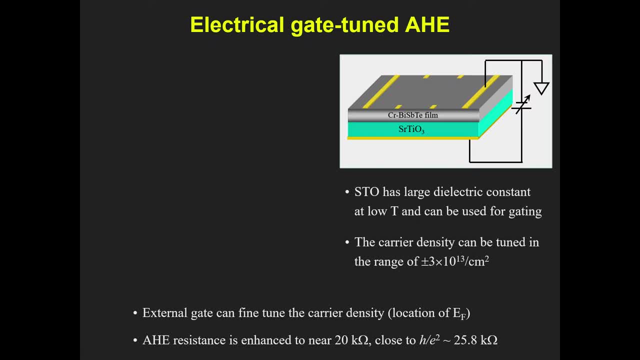 So now we grow this material on STO. STO is magical. It plays so many different roles together. It has a very large dielectric constant so we can use it as a bottom gate to inject a charge into the topological insulating film. 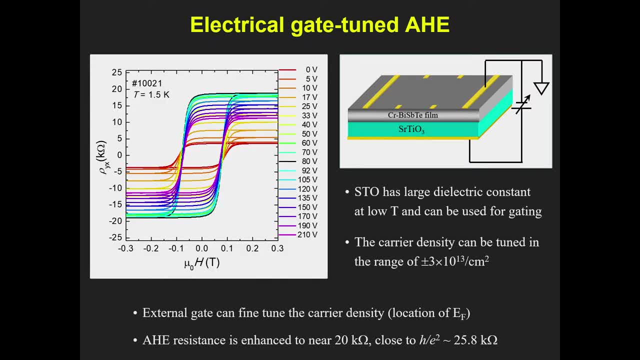 So still the same sample. In zero gate the anomalous Hall resistance is about 3 kiloohm. But as we increase to a positive gate the anomalous Hall resistance increases very rapidly And up to about 80 volts the anomalous Hall resistance is already 20 kiloohm. 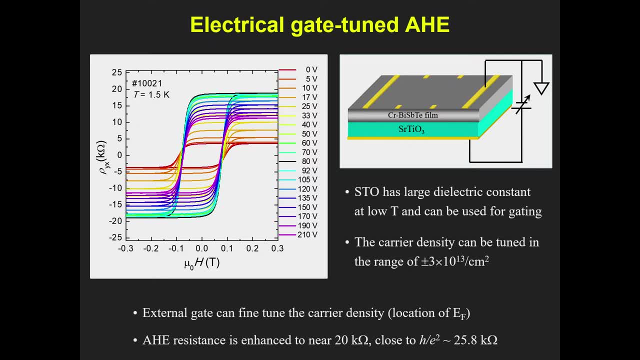 And upper bound is a quantized value. It's measured at 1.5 Kelvin. It's very close already. As we increase the gate voltage even further, the Hall resistance will drop. That's because now the Fermi level is tuning across the Dirac point. 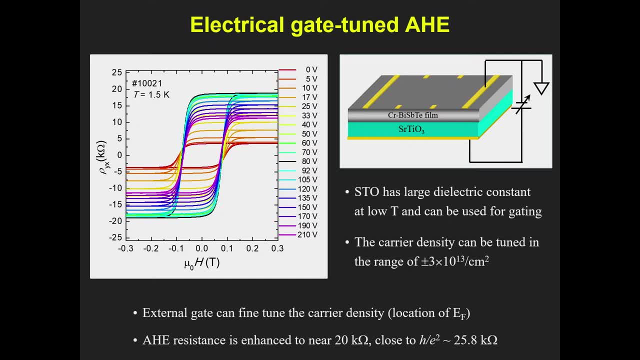 So more ball carrier gets in again. So when we get this curve, we know we are already in the quantum anomalous Hall regime. All we need is dilution refrigerator, But we don't have one. So we send these tempos and also our students. 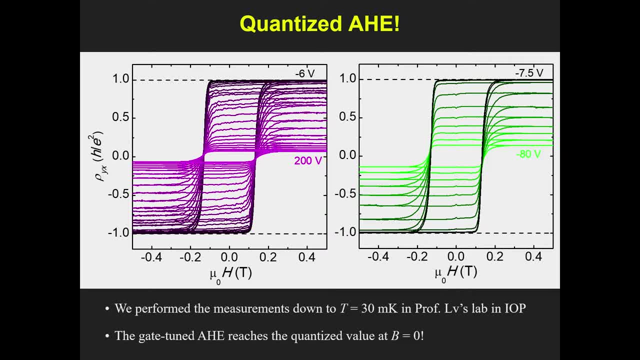 to Professor Lilly's lab in IOP and where we perform the measurement down to 30 millikelvins, And immediately we saw this beautiful quantized, anomalous Hall effect, just expected. in theory This is a gate voltage dependence. There's a narrow range of gate voltage. 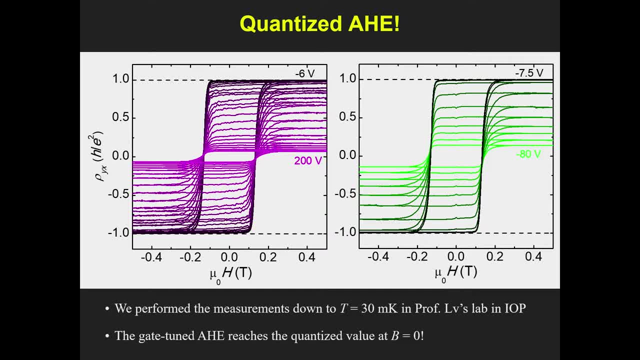 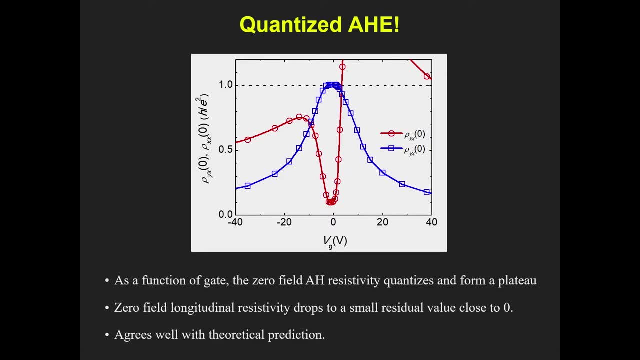 where the anomalous Hall resistance just stay at the quantized value, No larger, no smaller. So here's a summarized Hall resistance at zero magnetic field as a function of gate voltage, And you can see there's the quantized plateau for this range of gate voltage. 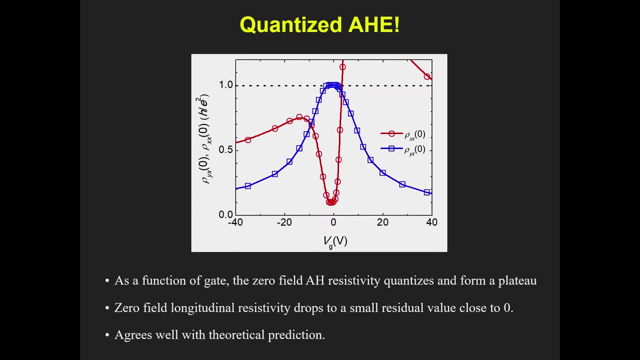 And meanwhile the longitudinal resistance at zero field also have this very sharp dip. that's also consistent with the quantum Hall behavior. where we have dissipationless edge state, We also apply a strong magnetic field to see whether there's any change to the quantum Hall effect. 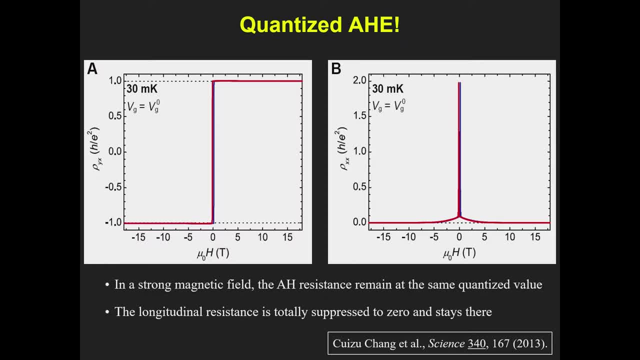 And in this measurement we have field up to 18 Tesla. You can see it's just a flat plateau all the way from zero field to 18 Tesla. Now we have new data: up to 60 Tesla in a pulsed magnetic field. 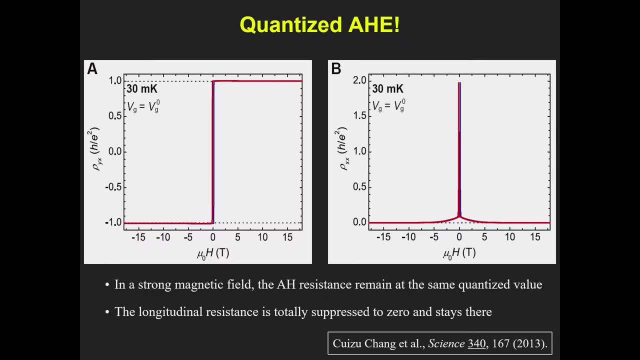 still the same plateau, no change at all. And in longitudinal resistance you can see at zero field it's already pretty small, but a strong magnetic field helps even better quantization And above 5 Tesla the longitudinal resistance is very close to zero. 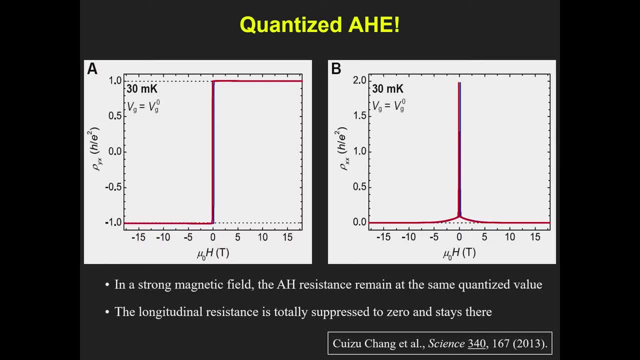 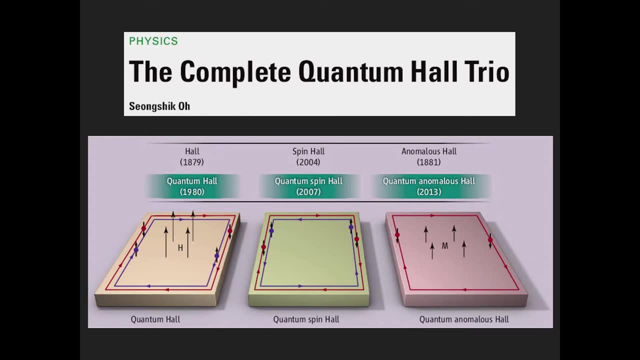 and stays there until 18 Tesla. So up to now we have very strong evidence that the quantum law of Hall effect is indeed achieved and later on is confirmed by many other groups, like Professor Kang-Wang mentioned, And of the papers published, there's a perspective by Sean Oh. 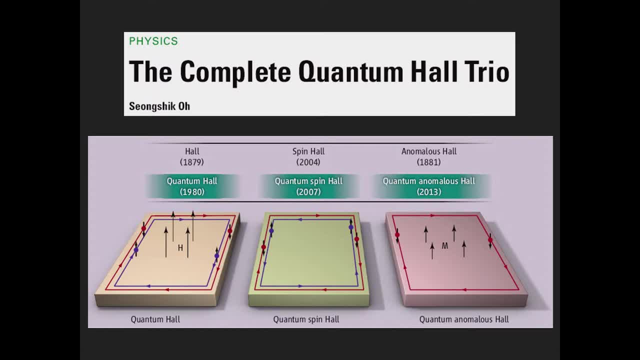 in Science called the Complete Quantum Hall Trial. It means the quantum Hall effect, the quantum spin Hall effect, discovered by Professor Molenkamp in 2007, and the quantum Reynolds Hall effect have both been discovered. In fact, these two effects are pretty similar to each other. 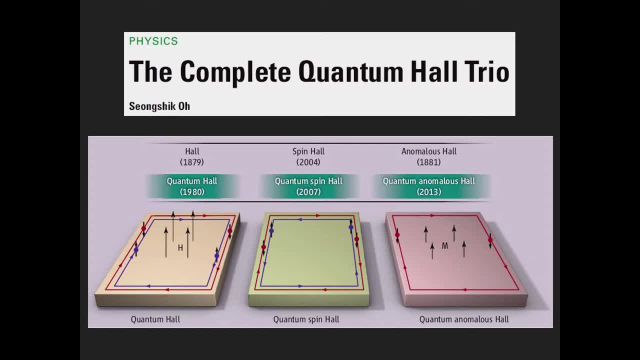 because time-rules of symmetry is broken. we have this chiral edge state And the quantum spin Hall effect is different because it preserves time-rules of symmetry and there is this helical edge state And recently we got interested in the quantum Hall effect. 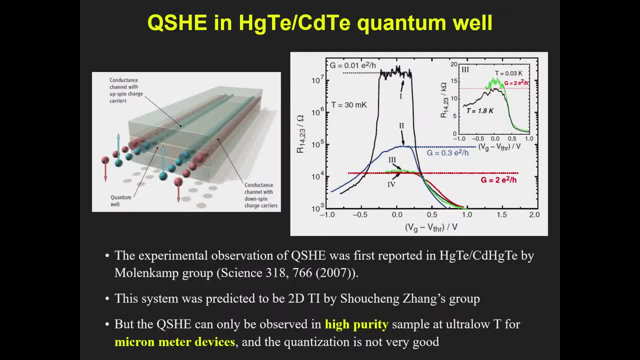 so we want to go back and see Professor Molenkamp's group. Here is the data, Here is the sample. It's a mercury telluride quantum wall structure which was predicted by Shoucheng Zhang's group to be 2D topological insulator. 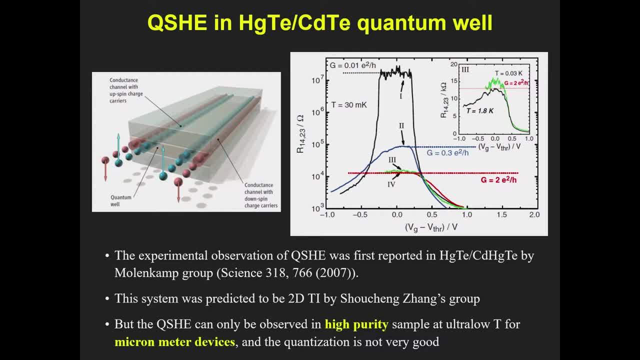 and which they have, this helical edge state. And here is the resistance as a function of gate voltage, and the broken line, the red line is the quantized resistance and the solid curve of the data. You can see, the quantization is not as good as the quantum Hall. 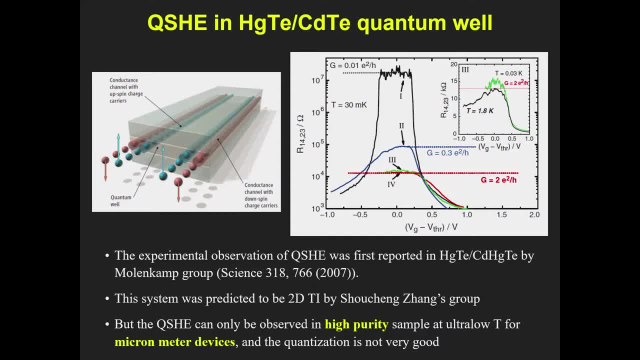 effect. but it's not surprising because when you have this helical edge state on the same edge, in principle it won't get scattered if the spin is always preserved. but as long as you have any spin defacing scattering mechanism, it will cause back scattering and destroy the quantization. 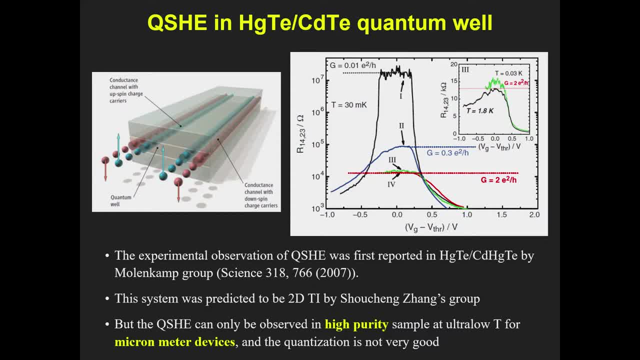 This is why, even for this kind of data, they need a very high purity sample, very low temperature and in very small devices. It's a very challenging experiment. The original idea of Chaoxing Liu is, if we start from quantum spin, Hall effect, put ferromagnet order into it. 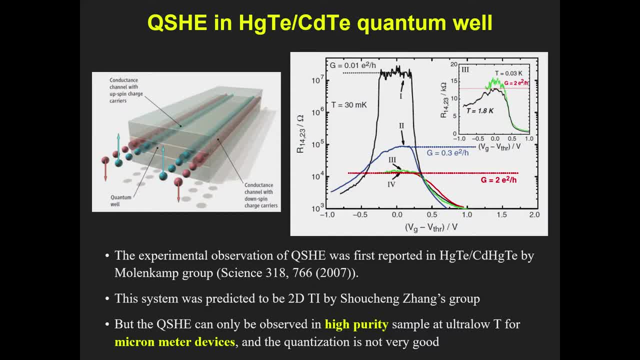 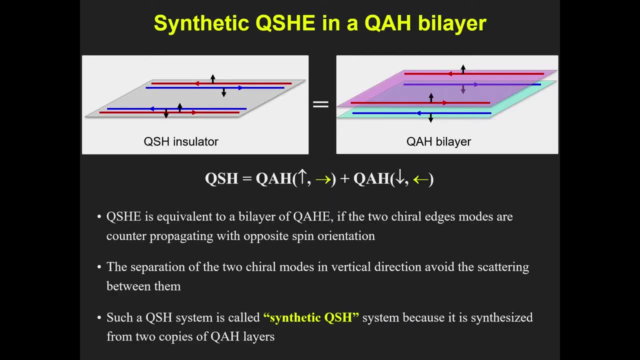 it may annihilate one of the edge states and change it into a chiral edge state and quantum normal Hall system. now we have very good quantum normal Hall effect. we thought can we go back to use this to construct a quantum spin Hall insulator? So if you look at this two diagram: 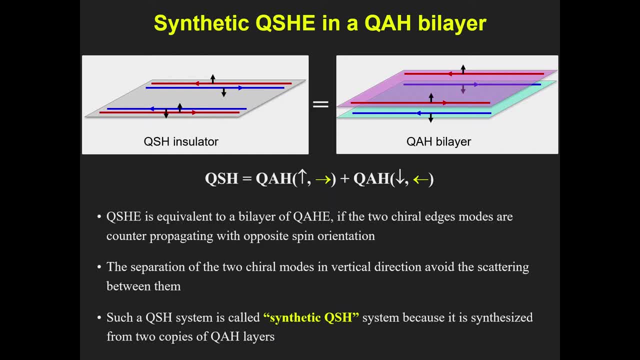 this is a quantum spin Hall insulator with a pair of counter-propagating edge states, and here we can actually use two quantum normal Hall insulators. if we can have opposite spin orientation and different momentum, we stack them together to form this binary system. then we can call it. 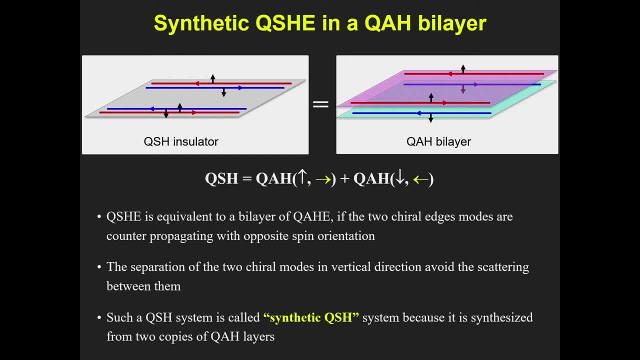 a synthetic quantum spin Hall, because from the symmetry point of view it's not a quantum spin Hall- temperature symmetry is broken. but from the transport point of view all the transport response expected for quantum spin Hall should be seen here. So this is why we call it. 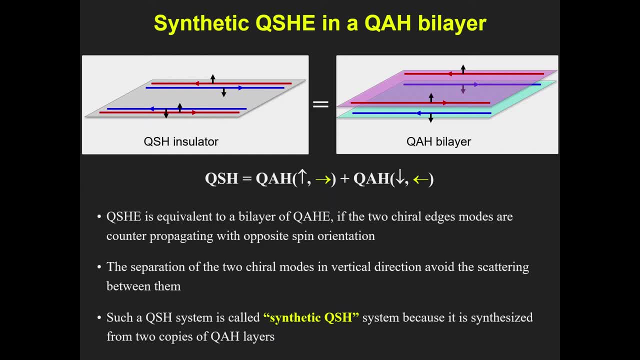 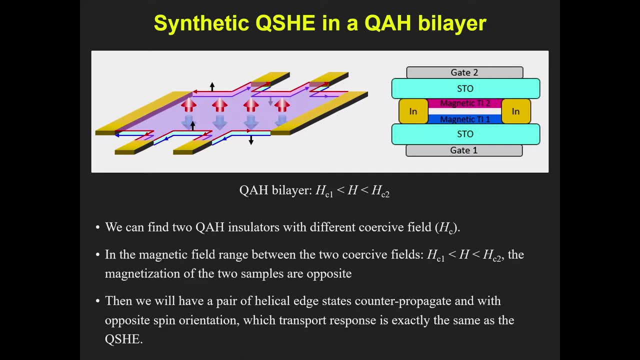 a synthetic quantum spin Hall system. so this is a schematic structure for the device. if we can have two quantum normal Hall with opposite spin orientation and opposite momentum of the edge state, they may realize this is a synthetic quantum spin Hall. so what we do is we find two magnetic topological insulators. 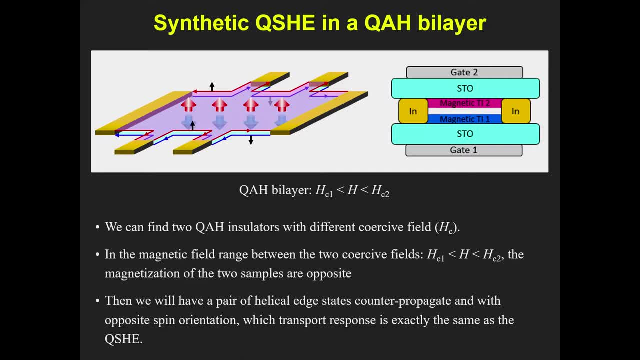 with various different coercive fields. so in the structure we have two magnetic topological insulators, one magnetic field. they are aligned together, but with the reverse magnetic field one of them is flipped first. so in this regime we will realize this structure. so basically two quantum normal Hall systems. 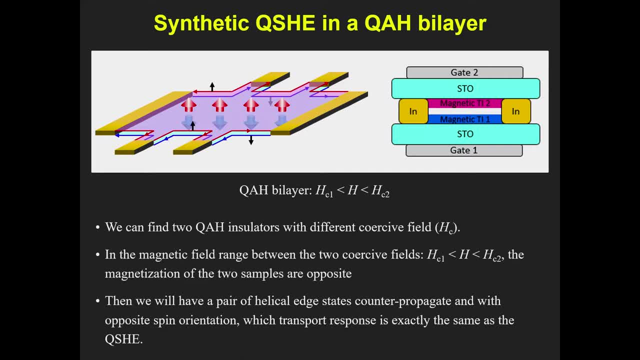 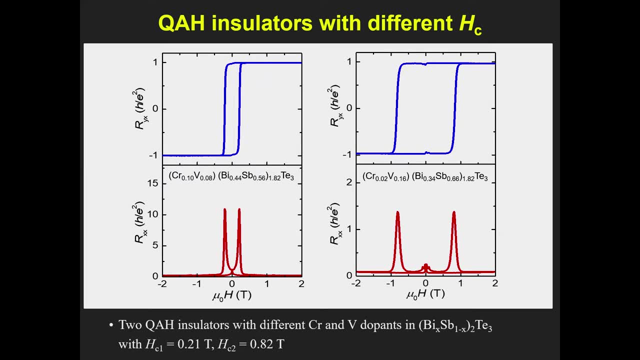 stack together to form this bilayer. then the next question is: how do we control the coercive field of a magnetic TI? so in recent years it has been found that chromium and vanadium doping into bismuth antimetalluride by mixing them together. 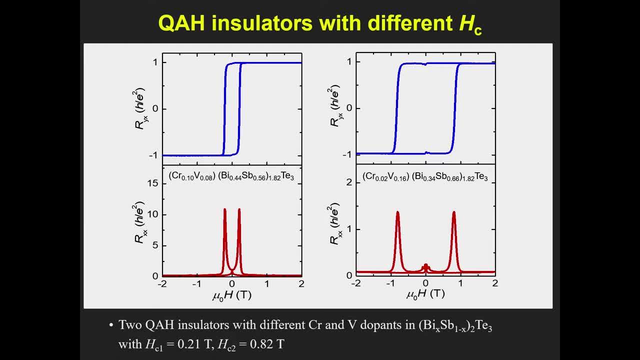 we can actually tune the coercive field almost continuously. so in this experiment we have a chromium rich sample which has a smaller coercive field about 0.2 tesla, and the vanadium rich sample which has a coercive field around 0.8 tesla. 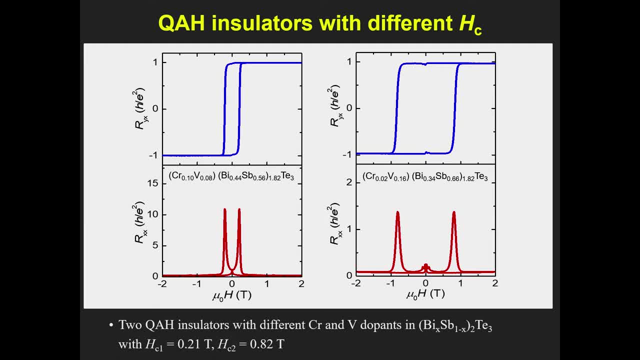 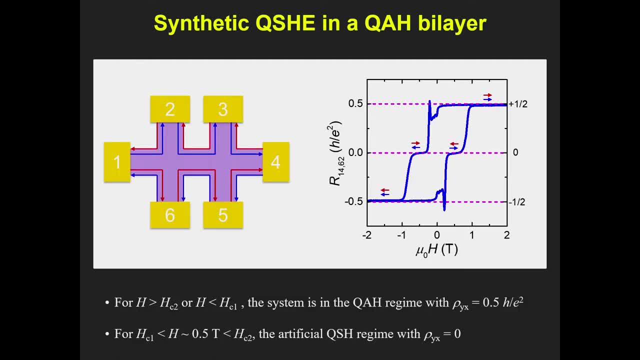 they both have very nice quantum normal Hall effect. so if we stack them together to form this bilayer somewhere in the middle around 0.5 tesla. so what we found? experimentally we form this bilayer, cut it into a Hall-bar geometry and measure the Hall effect. 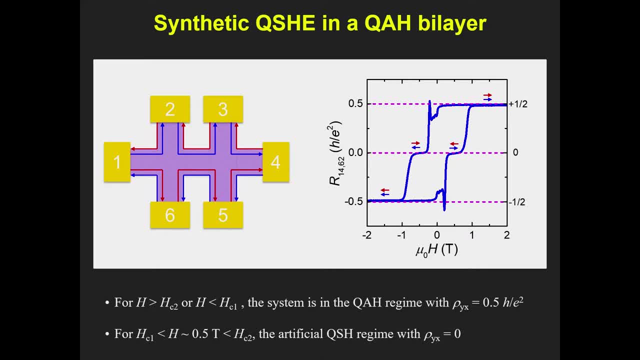 apply current from 1 to 4 and the Merus voltage from 6 to 2. you can see in strong magnetic field. it's very simple: it's two copies of quantum normal Hall which give you this half plateau and then we reverse the magnetic field. 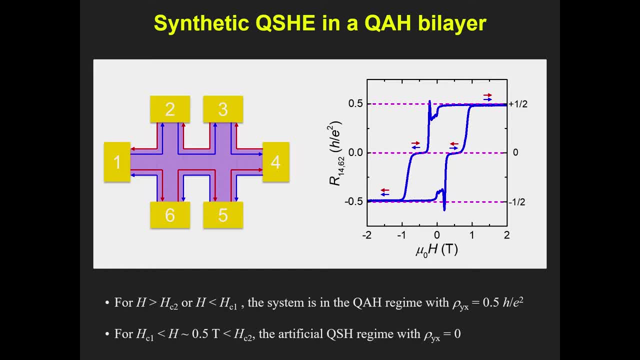 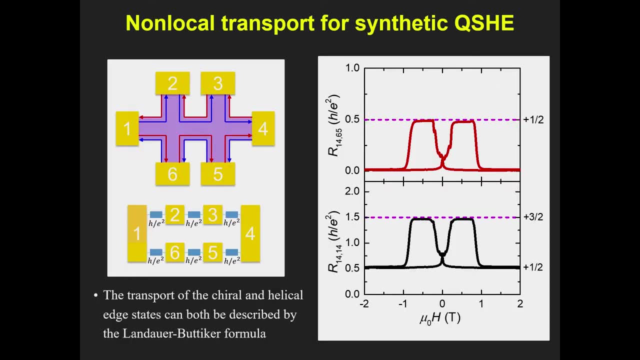 in the mid field regime we will have this synthetic quantum spin Hall and when the two Hall channels cancel each other, we have this zero plateau. that's pretty easy to understand. then we also did other non-local transport or multiple terminal transport. for example, we can measure 1,, 4,, 6,, 5. 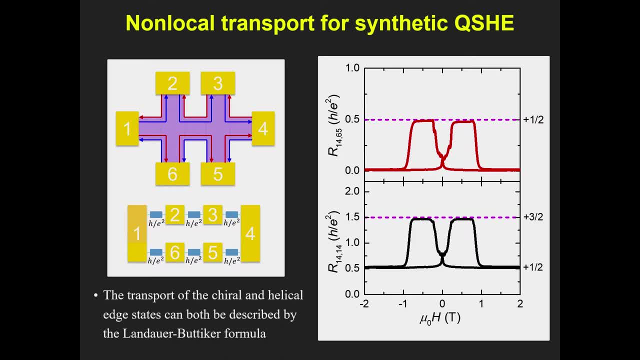 is that simple: four terminal measurements. and in the intermediate regime, if it's in the quantum spin Hall regime, the physics is very simple: between any neighboring contact there will be a quantum resistance. so for this, 1,, 4, 6, 6, that's the diagram. 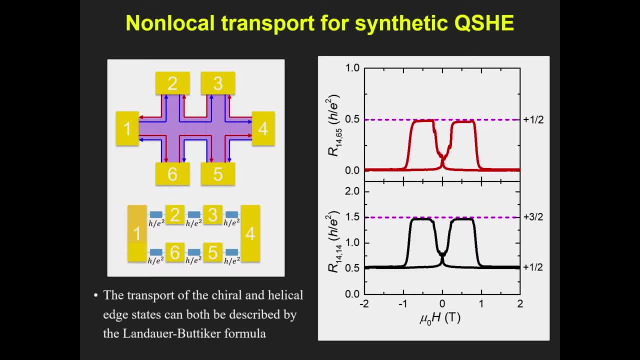 where we pass current from here to here and between them there's a quantum resistance. but because the device is symmetric, the current will split into two, so you expect to see a half plateau, which is exactly seen here. we can also measure two terminal resistances: 1, 4, 1, 4. 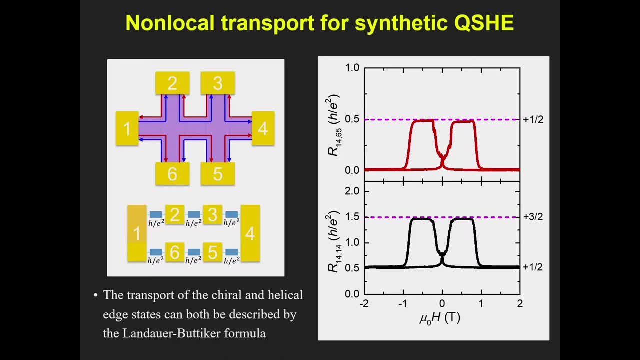 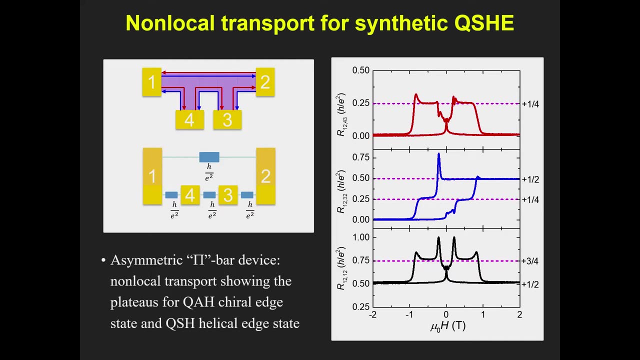 there are three quantum resistances on each side, so the total resistance between them can be measured here. so it's a very robust, nice quantum spin Hall response. we also cut the sample into a pi bar junction, so now it's asymmetric. so that's equivalent electrical diagram. 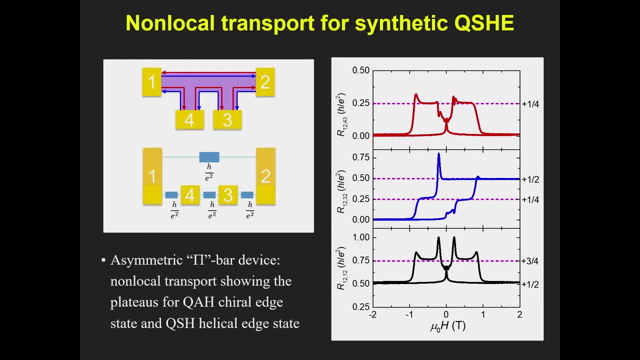 again in the intermediate regime we will find 1,, 4,, 1, 5, 3, 4 quantum resistances, just expected from Landau-Budecker formula for helical edge transport. so up to now, what we do is only to simulate the quantum spin. Hall state. 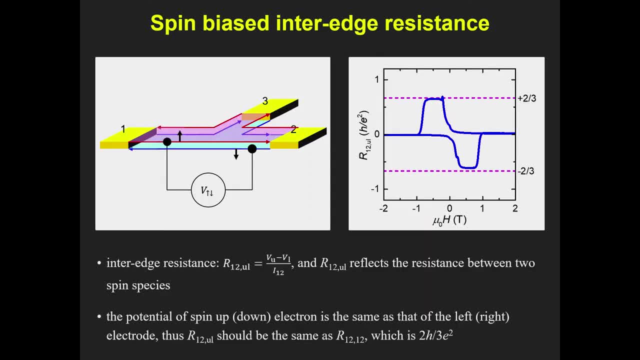 of the quantum anomalous bilayer. but this bilayer structure can also allow us to do more than that. for example, we can now measure the interlayer or interedge resistance between the upper edge and the lower edge in the quantum spin Hall regime. these two edges will have 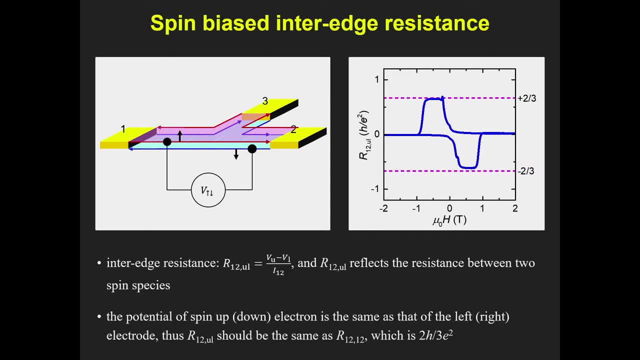 different, opposite spin orientation. so this resistance between two of them will be spin biased, namely it's a resistance between two spin species and because edge state is spinless, the potential here is the same as one and the potential here is the same as two. so the resistance between them is also quantized. 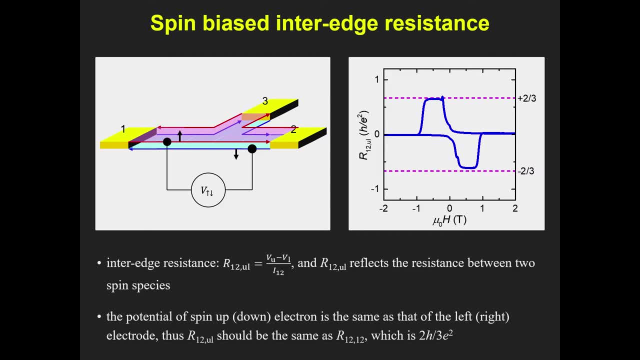 so now we are having a quantized spin, biased interedge resistance and experimentally we see this two-thirds quantum resistance. it depends on how many electrodes you add on the other side of the device. so this is one project we have completed recently. we think maybe based on this. 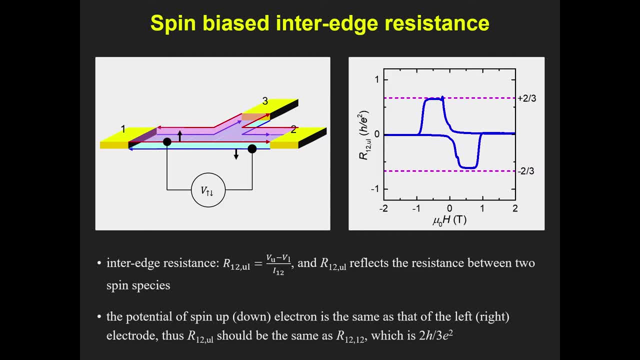 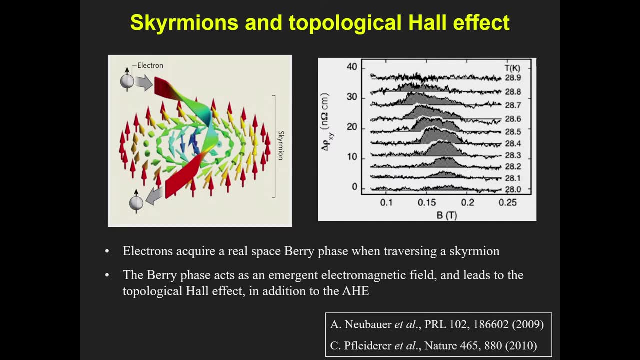 we can get more and more interesting devices and potentially some applications based on the quantum norm Hall effect. up to now, when we talk about the topological order, it's a non-trivial topology in momentum space, in the band structure. but we know, actually in magnetic materials there could also be. 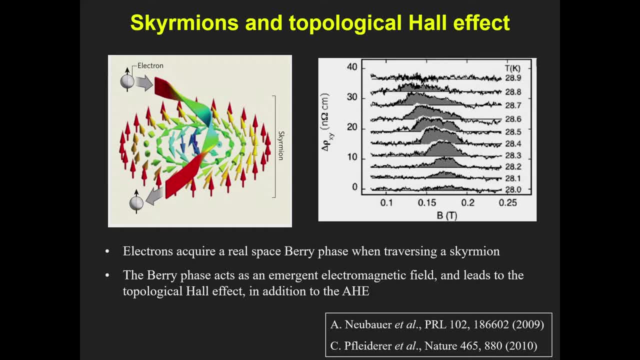 non-trivial topology in real space, such as a skirmish, which is a topological object formed by local moments. so when an electron travels through a skirmish, it will pick up a barrier phase because the exchange coupling between the acting electron and the local moment, this barrier phase will act. 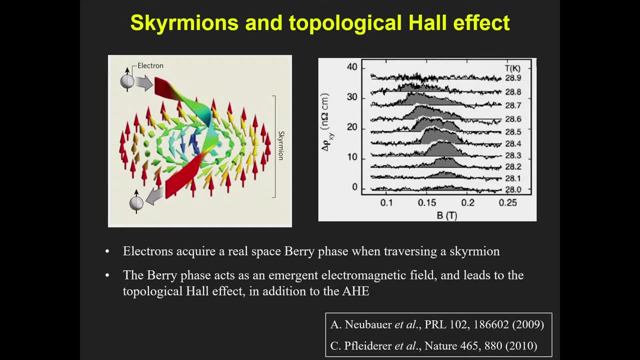 as an emergent electromagnetic field, so it will generate its own Hall effect, which is usually called a topological Hall effect. the experimental signature is a broad hump on top of the anomalous Hall effect, so this is well known for many different skirmish systems and recently. 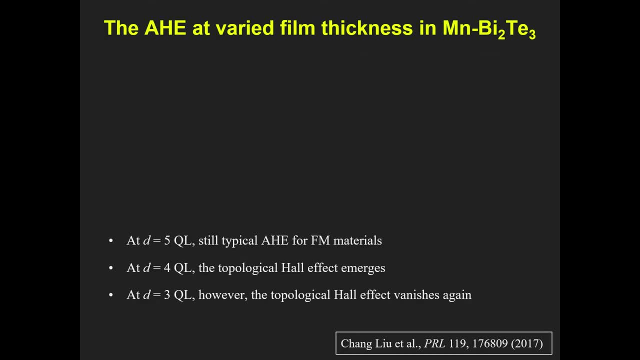 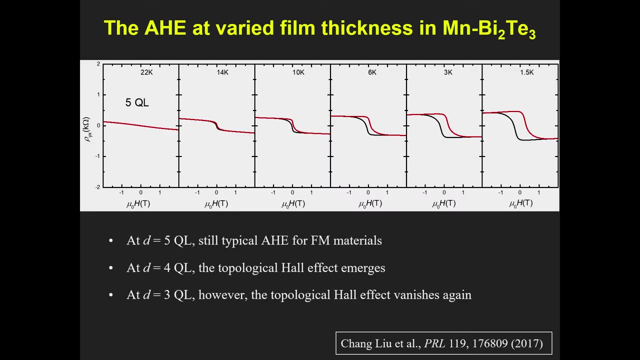 we found that also in magnetic topological insulator the material system is manganese doped bismuth telluride. actually we have studied so many different manifestations of magnetic elements and topological insulators. the reason we want to understand this material is because the anomalous Hall effect 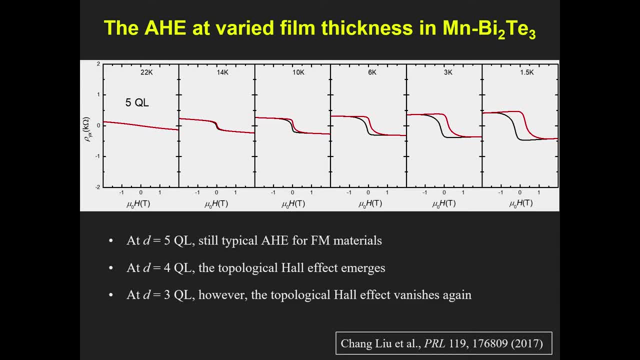 has the opposite chirality from the chromium doped one. so actually we want to achieve quantized anomalous Hall effect with a different chirality, but we haven't done that yet. however, we found something quite interesting. so this is a five quintuple layer of five nanometer thick. 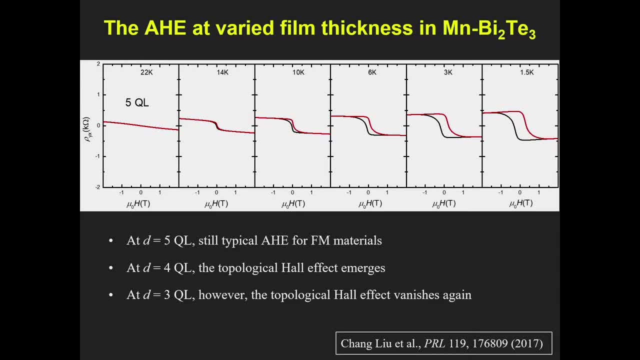 manganese doped bismuth telluride which has an anomalous Hall effect. but when we reduce the thickness just a little bit by one unit cell to four quintuple layer, and immediately we saw this very pronounced signature of the topological Hall effect found in skirmish systems. 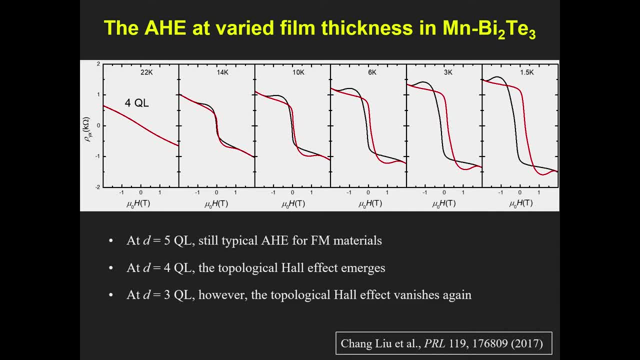 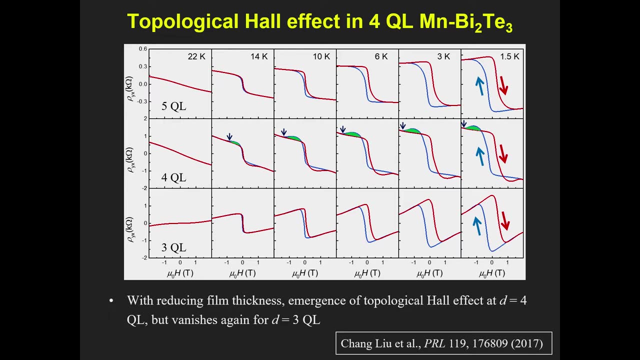 then we reduce the thickness again by one unit cell to three QL and the topological Hall effect is gone. it returns to the very simple, anomalous Hall effect. so in this figure I show the three samples together. it's the same material but just different thickness. 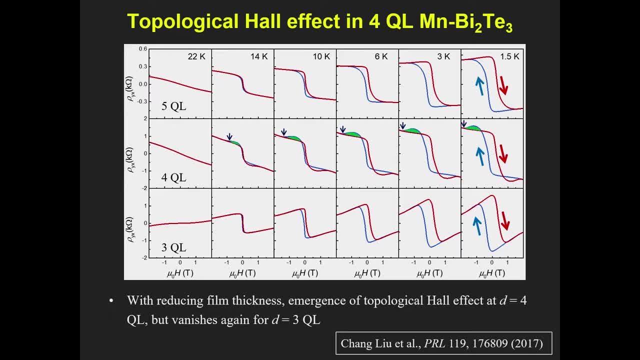 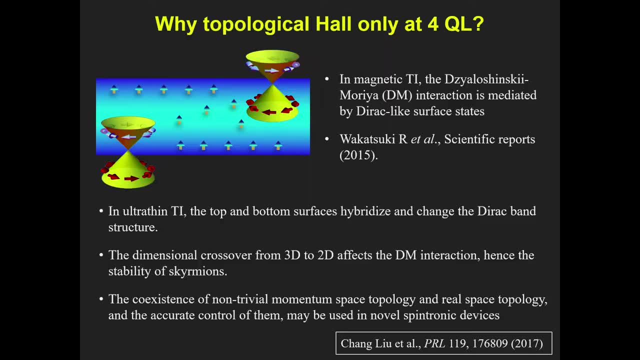 and you can see the creation and annihilation of the topological Hall effect. so somehow the topological Hall effect is only stable at this particular film, thickness four, quintuple layer. so then the question is, why? why topological Hall effect only at this thickness? we have a simple theory about that. 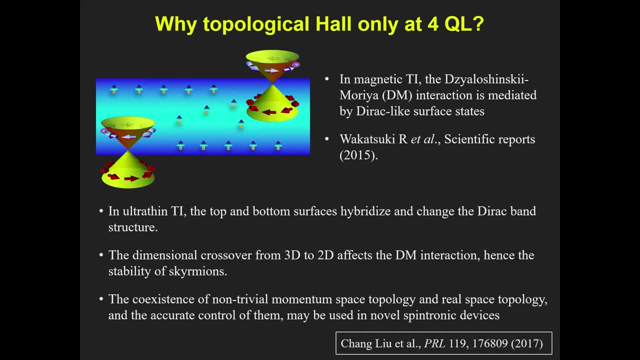 and also some numerical simulation in this paper. the basic idea is: in topological insulator, the DM interaction, which is responsible for the creation of skirmish, is mediated by the topological surface state, and when we make the topological insulator very thin, the topological surface 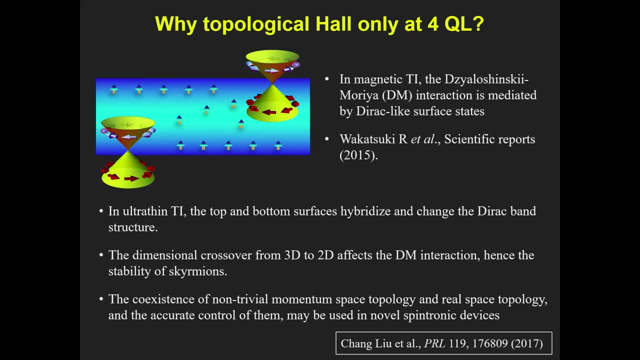 can actually hybridize with each other and that will change the band structures, for example, open a gap at the direct point and we know for this family of material there's a transition or crossover from a 3D topological layer with decoupled surface state. 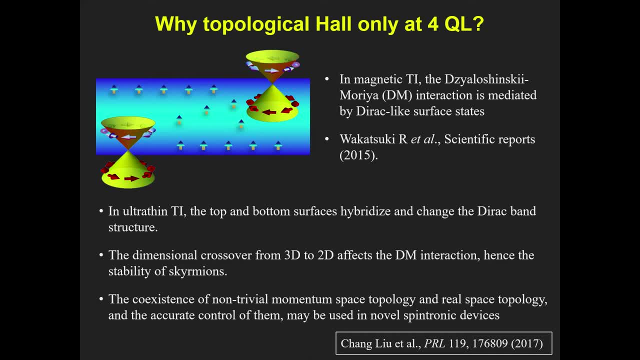 to 2D with strongly coupled surface state, and that occurs roughly around a quintuple layer. so what we believe is happening here is that in this dimension of crossover regime the change of band structure will have a favorable energy scale to stabilize the skirmish. so in this particular thickness, 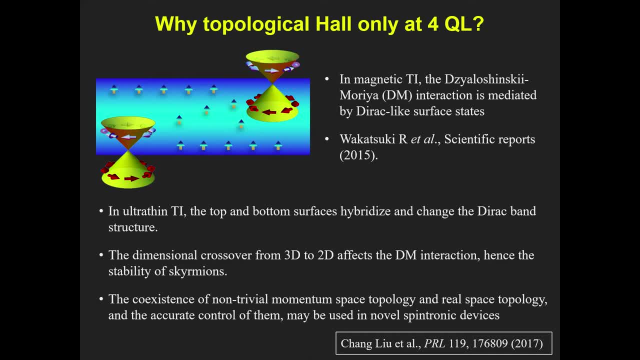 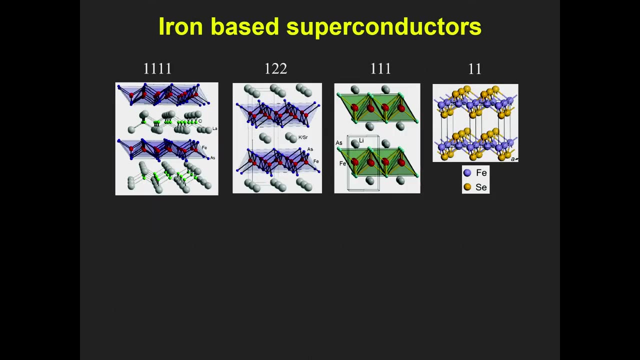 we will have the coexistence of non-trivial momentum space topology and also real space topology, and we can tune it accurately by changing the film thickness. so we think that may also have some application in spintronics. so now I've reached here to a totally different topic. 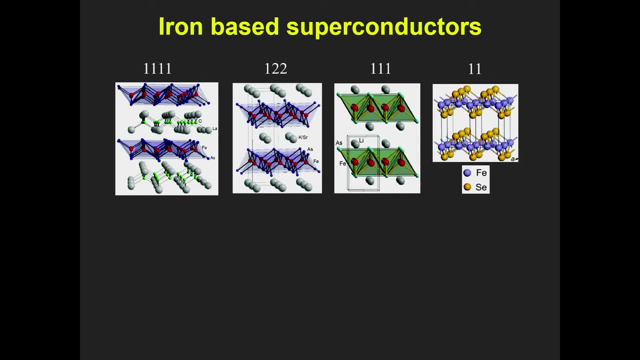 it's about ion-based superconductors. so these are the four families of commonly studied ion-based superconductors, and the most simple one is ion selenide, what we call the 1-1 system. it's just ion selenium forming a layer by layer structure. 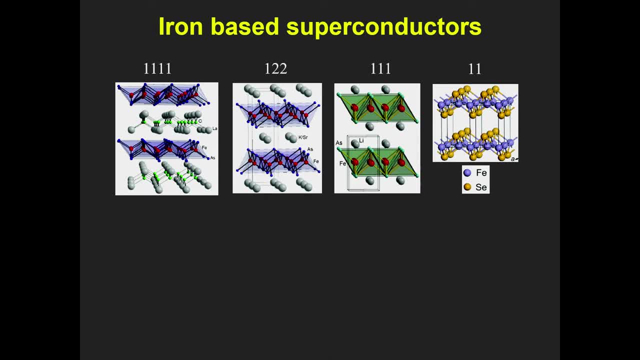 so when sequence groups saw this, they said we must be able to grow this by using MBE and study its property by in situ R-pass and STM. so they treat this as a model system because it's so simple to test the mechanism for pairing in ion selenide. 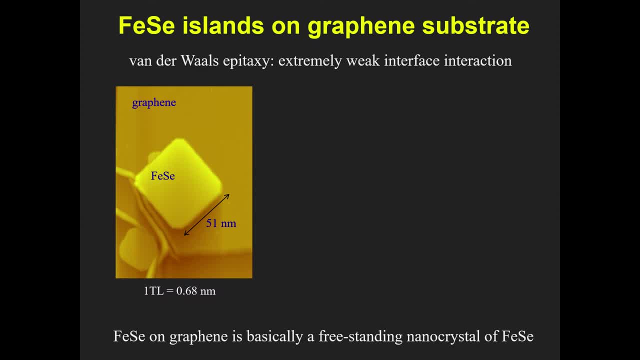 and this is their first trial. they want to grow this material on graphene because it's very easy. it turns out the coupling between ion selenide and graphene is very weak. the bonding between them is van Waals, so the ion selenide just grows into a tiny piece. 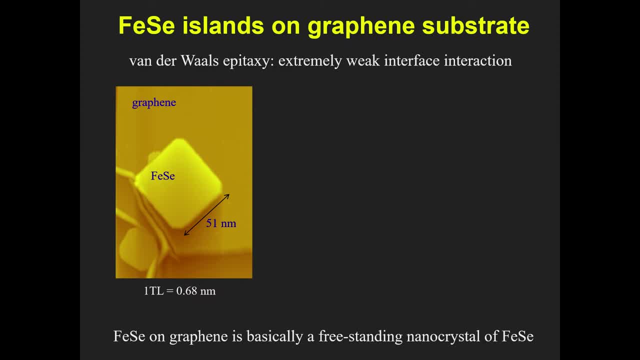 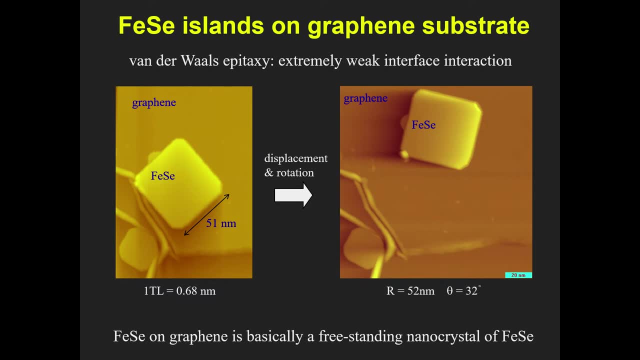 of nanocrystal on the top to show you how weak the bonding is. they can actually use the STM tip to move this island as a whole and you can see they can just push it a little bit from the edge and even rotate it a little bit. 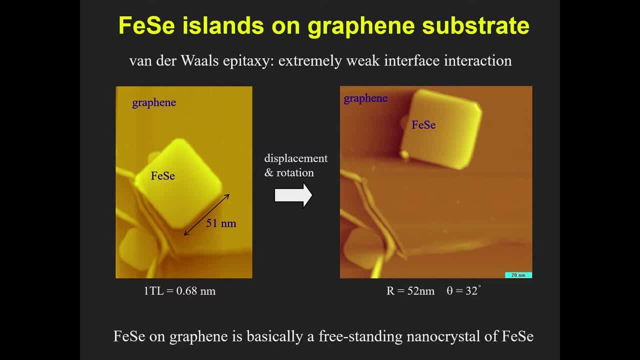 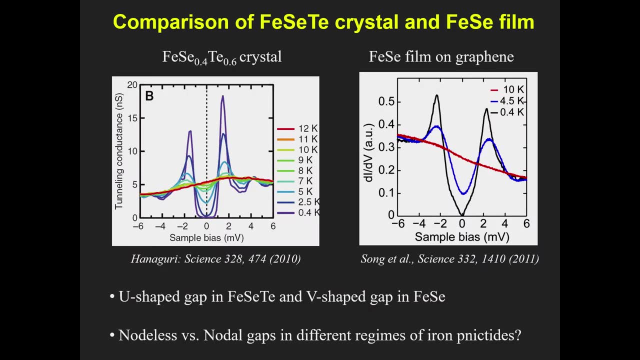 it's the same island. you can see there's sort of a marker over here, but this one has the best crystals quality for ion selenide at that time, so they can perform very high quality STM experiments that already show some very interesting results. it's the first paper they published back in 2011. 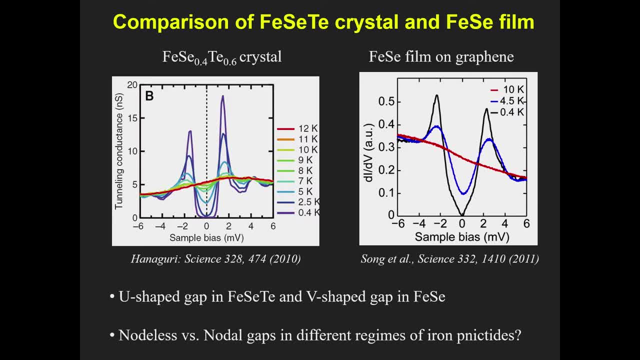 they studied the DIDV curve on this ion selenide film on graphene and they saw this V-shaped tunneling spectrum, meaning the gap is most likely nodal. a year later than that, the Hannibal group in ion selenide telluride single crystal. 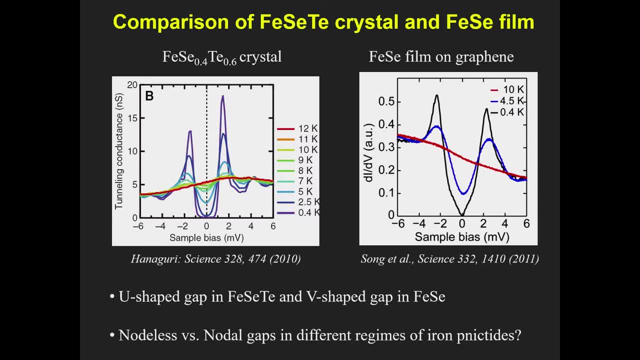 they found this very nice U-shaped gap. both results have been reproduced by other groups, so that's true. somehow, by just increasing the tellurium content, you can change the material from a U-shaped gap to a U-shaped gap, maybe from a nodal superconductor. 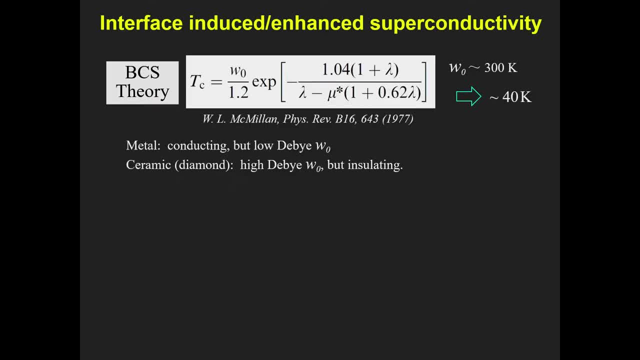 to a nodal superconductor. that's already quite interesting, but not enough for Qi Kun. actually, back in 2008 he already proposed that maybe we can use an interface to find a generic approach to find a high Tc superconductor. the idea is pretty simple. 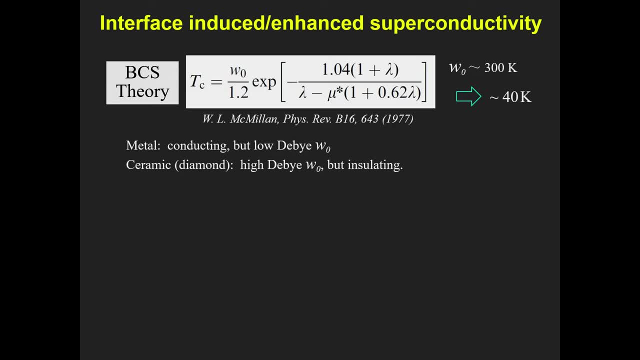 and naive. if you just look at the Macmillan formula for BCS, superconductor Tc is determined by the bifrequency strength. for most metallic superconductors it's conducting, but usually the temperature is very low. if you want to have high temperature to enhance Tc, 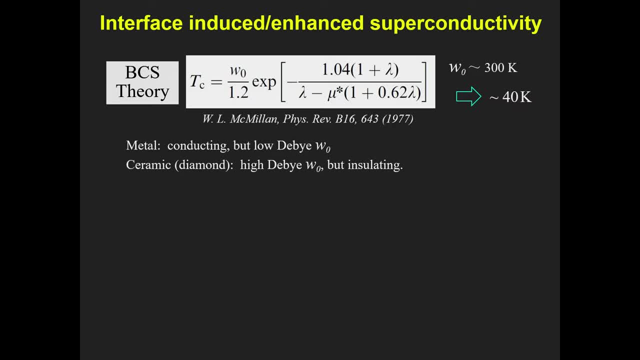 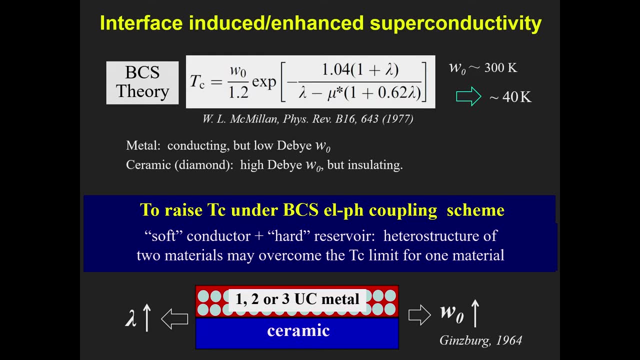 then you better have ceramic or very hard material like diamond, but most of these materials are insulating. so Qi Kun's idea is: can we combine these two different materials, a soft metal on a very hard substrate? so in that case, instead of conducting from the metallic sample, 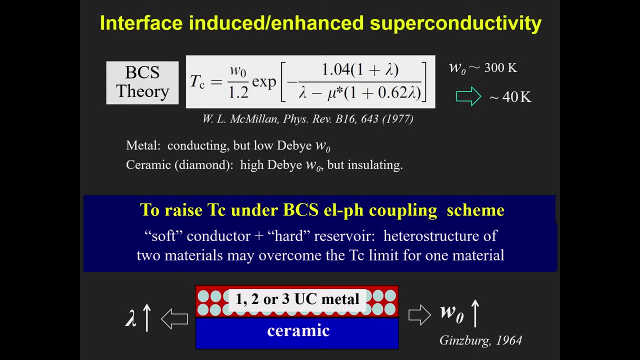 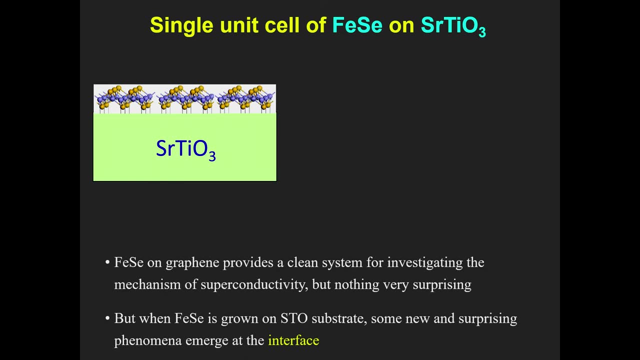 but very high the bifrequency from the substrate and probably very high, very strong electrophonal coupling at the interface, then you have the advantage of both cases and probably can enhance Tc. that's a naive thinking, but he applied it to ion selenide on STO. that works magically. 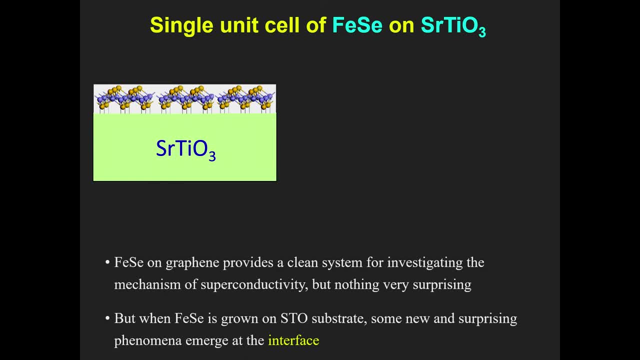 so he tried to grow a single layer of ion selenide on STO substrate and he succeeded. you can see in the middle already that the growth dynamics are very different from that on graphene substrate. on graphene, the sample wants to form this tiny free standing island. 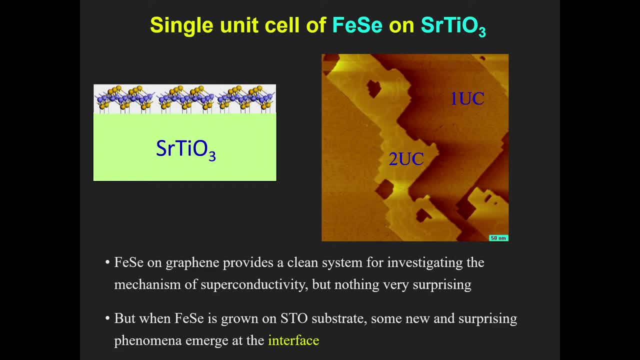 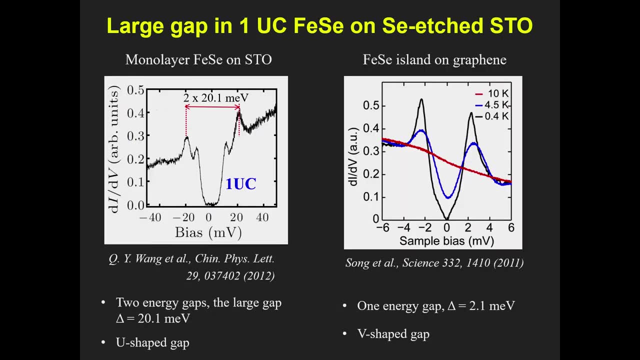 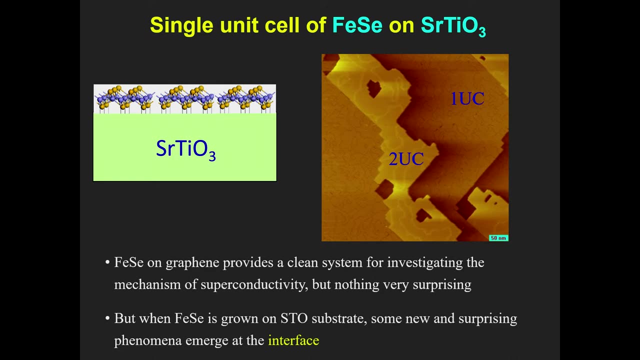 but on STO substrate the film growth is layer by layer. that already tell you the bonding between the film and substrate is quite strong. then he performed STM experiment on the first layer, the monolayer. actually he can have different layers, one or two different unit cells. 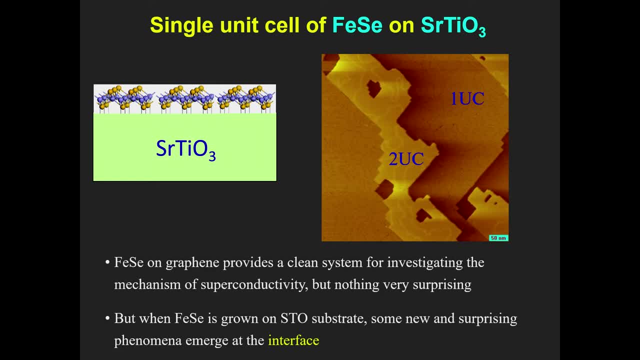 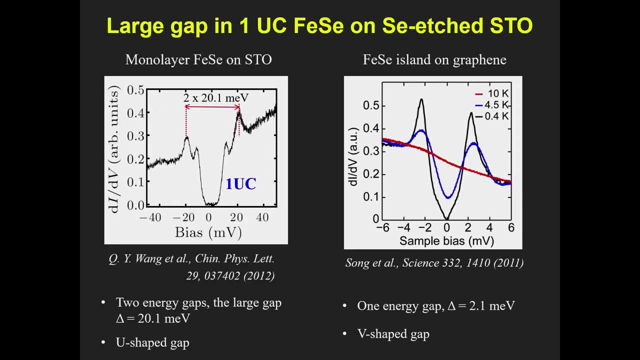 but it turns out only the first layer, the first unit cell, is superconducting and when he performed STM experiment you can see the gap size is about 20 mEV. it's a huge gap, remember. in this island of ion selenide on graphene the gap is only about 2.1 mEV. 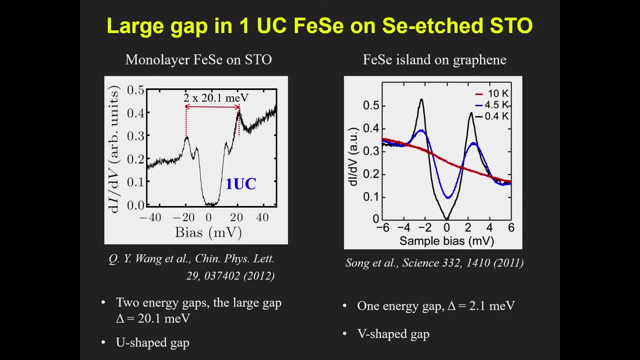 so somehow there is 10 times enhancement of gap size. that's the first finding. the second one is now: in this one unit cell ion selenide on STO, the gap has a U shape, which again becomes a noteless superconductor. so these two big differences. 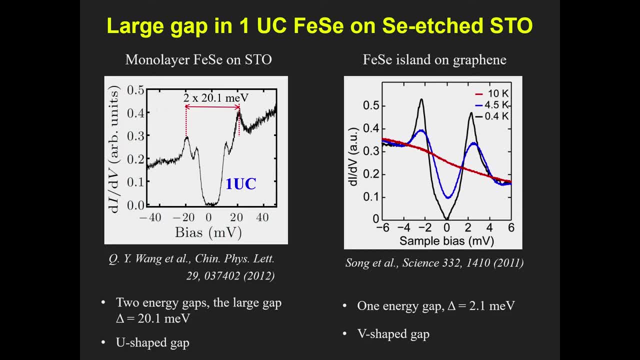 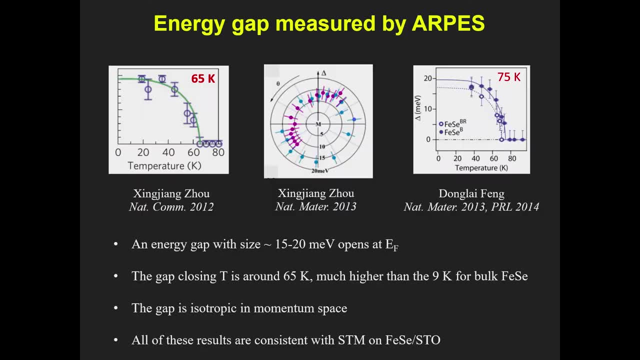 tell us that somehow ion selenide on STO is totally different from this free standing ion selenide island. all of these discoveries by STM have later on been confirmed in our experiment. for example, this is the work by Xinjing Zhou's group and also Donglai Feng's group. 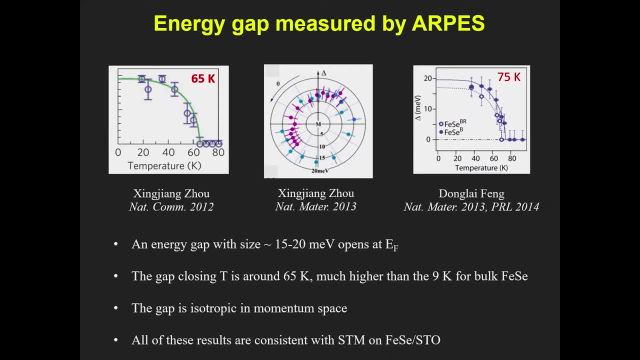 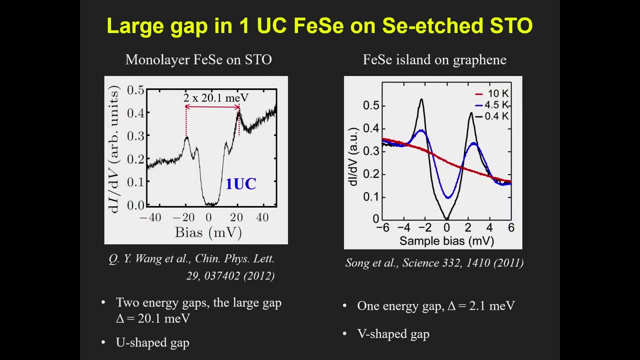 in this where you can see there is a gap at around 65 to 75 Kelvin. so if you compare this gap size, it increased by 10 times. and the Tc of this ion selenide is about 8 Kelvin. so by a simple counting you will expect: 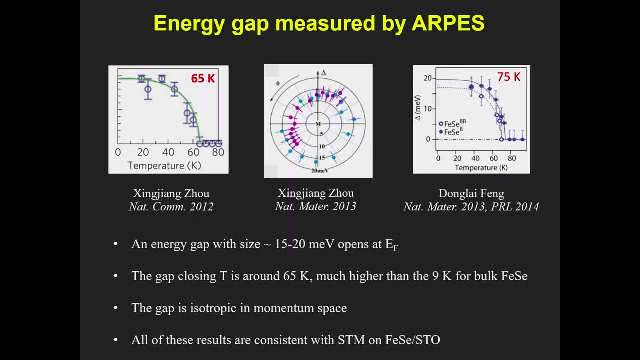 something around 70 Kelvin Tc, and that's what exactly observed by RPAS, and also the gap size in both experiments between 15 to 20 mEV. that's also very conditional with STM. moreover, Xinjing Zhou's group did the momentum space dependence. it's highly isotropic. 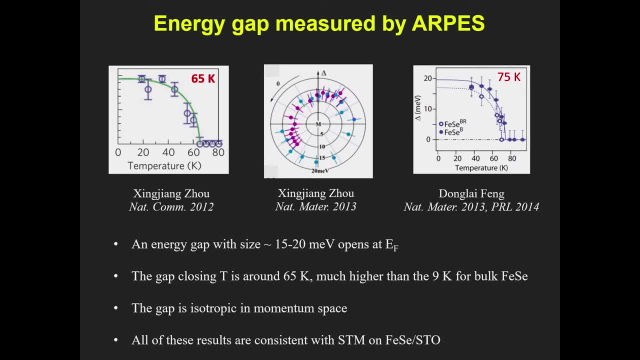 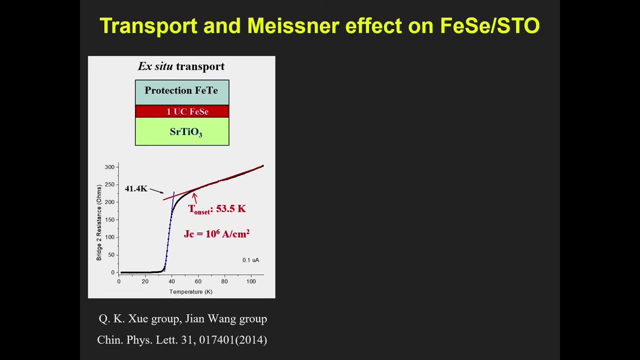 meaning it's not nodal. so all of these three results are consistent with STM. but there is always a question: are these gaps really superconducting gaps? many mechanisms can give you a gap. in order to confirm it's a superconductor, you have to perform transport experiments. 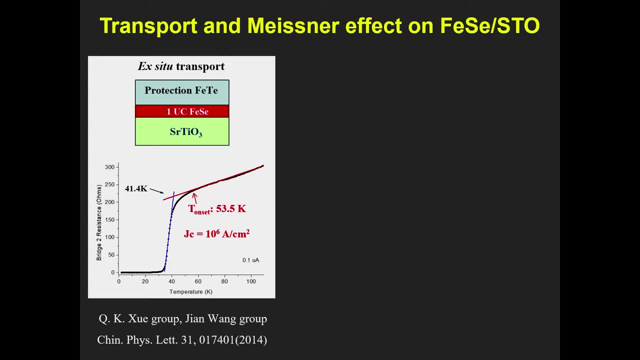 to show zero resistance and a mass effect to show the expulsion of flux. but these are much harder experiments because STM and RPAS are in situ in the UHV environment and do the measurement directly. but for this bulk measurement we have to take the sample out of the UHV environment. 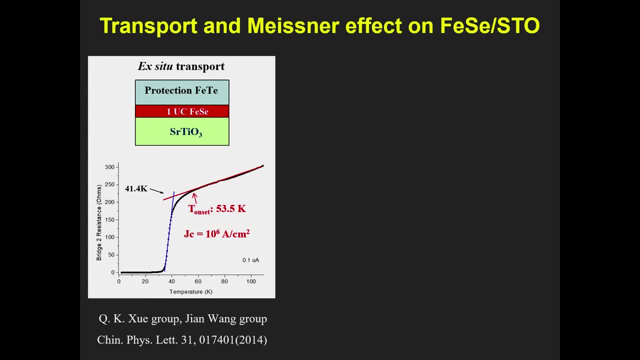 so that's much harder and we need to protect the sample. so in the transport experiment we use an ion telluride which is an insulator and can grow episectly from the ion selenide fuel and protect it and do the transport measurement. you can see the on-site temperature. 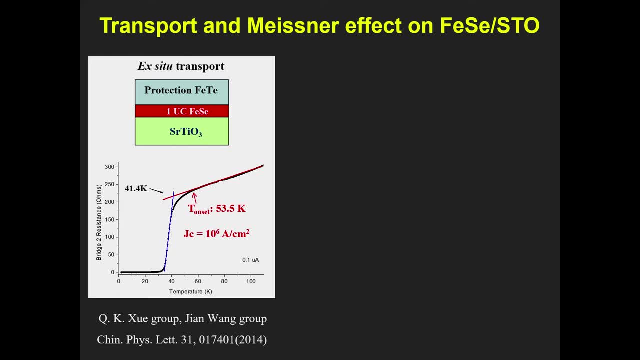 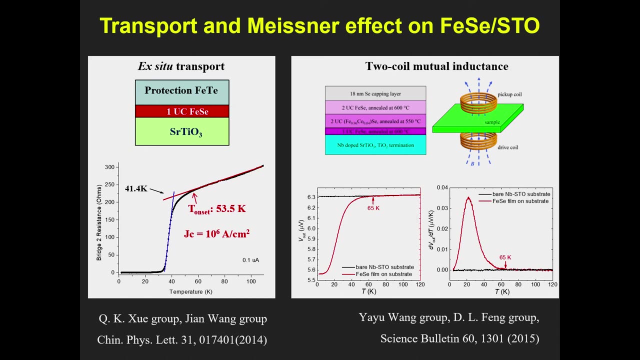 of the resistive transition is about 53 Kelvin or something like that, so it's definitely a superconductor and a high-temperature superconductor, although the Tc is slightly lower than what the gap measurement tells us. this was done by Jianwang's group. 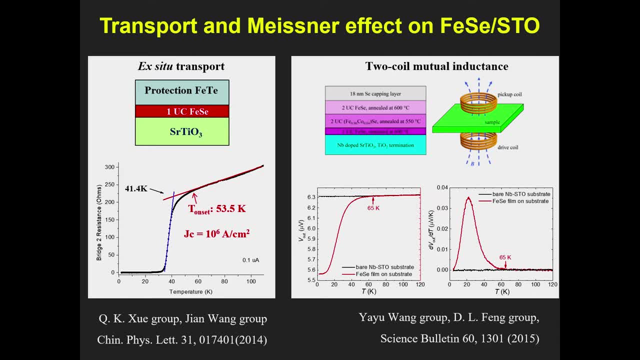 in PQ, my group collaborated with Donglai Feng's group. we also grew a monolayer of ion selenide. the difference from a Qikun sample is now: the film is grown on metallic STL substrate, which is much easier to prepare and has much better quality. 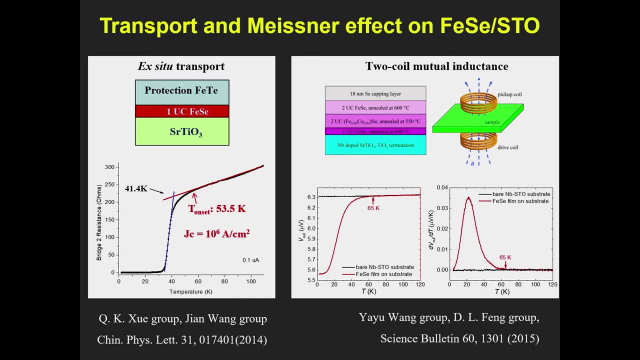 but because this is a mass effect measurement, we can use a metallic substrate. so we put this sample in a 2-quo mutual inductance measurement system. basically, we measure the screening by this superconducting film and the black curve is the data of a pure substrate. 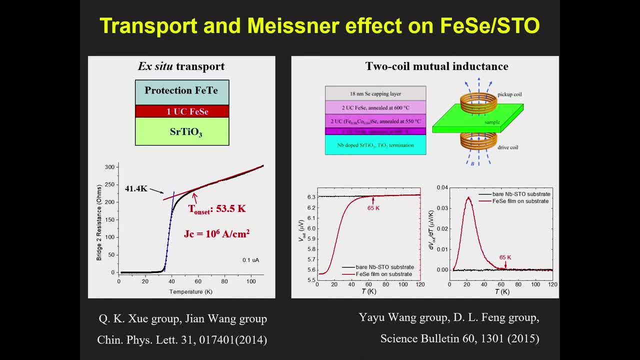 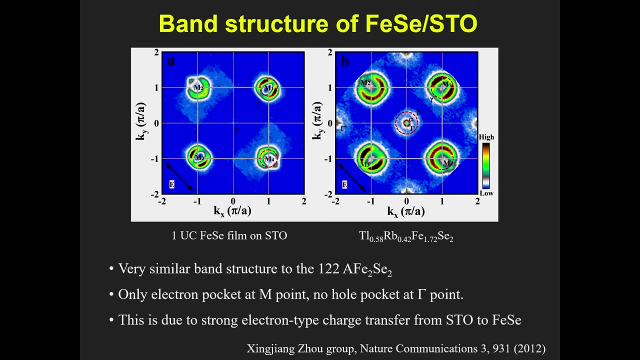 without anything. it's nothing happening and the red curve is with this one monolayer ion selenide on the substrate and immediately you can see the screening starts from somewhere around 65 Kelvin, which is very consistent with the RPAS measurement of the gap size. 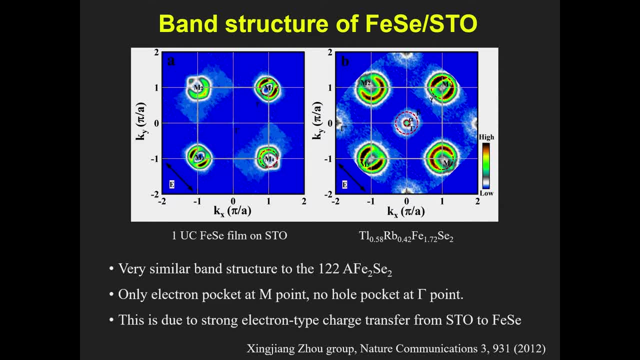 then the next big question is why the Tc is so high in this monolayer ion selenide on STL. then we need to look at the band structure carefully again. this is work by Xinjiang Zhou's group where they measure the monolayer ion selenide. 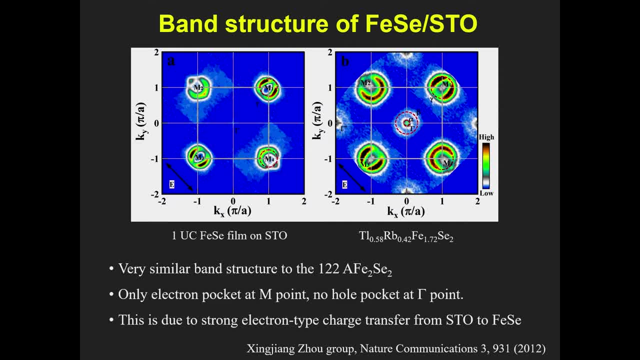 on STL the band structure becomes really simple. there are only two nearly degenerate electron pockets near the M point and at the zone center gamma point. there is nothing like Fermi surface pocket as seen in bulk ion selenide. the reason, we believe, is because there is a very strong charge transfer. 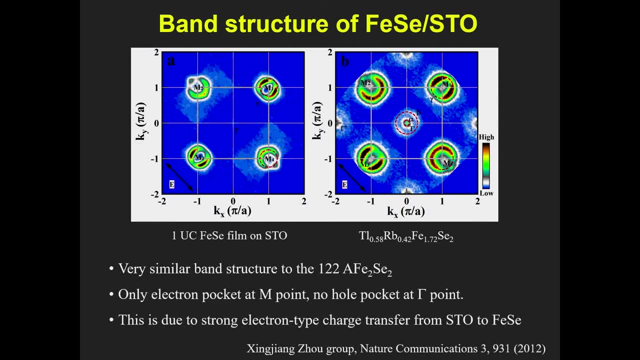 from the substrate, from STL to ion selenide, which will sink this whole type of electron pocket. at that point that will help to enhance Tc to somewhere around 30-40 Kelvin, as people observed in other ion selenide systems. but that's not enough. 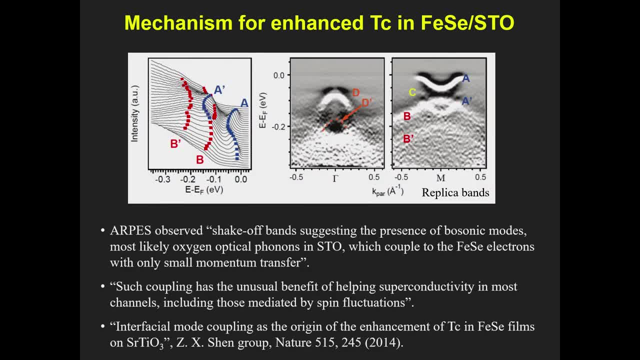 to explain this 65 Kelvin superconductor. two years later, Xinjiang Zhou's group also performed very high resolution ARPAS measurement on this ion selenide, on STL. they found something very interesting and I think they summarized very nicely in their title of the paper. 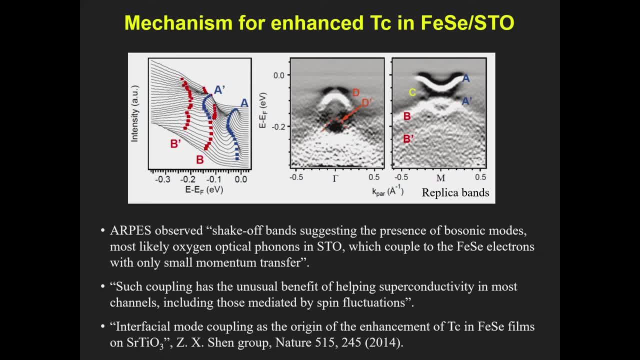 they conclude that the interfacial mode coupling is the origin of the enhanced Tc in ion selenide fuel. basically, in this ARPAS measurement they see the replica bands for most of these conduction valence bands like A to A prime, B to B prime. 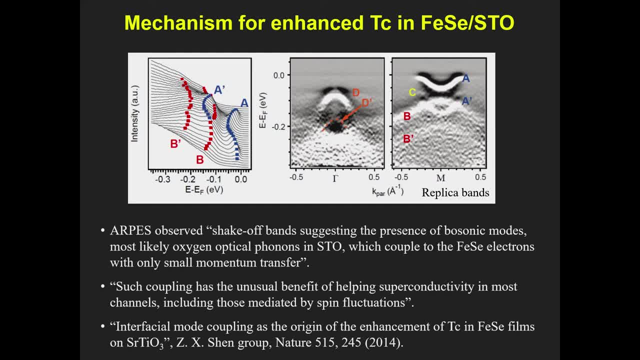 and that's the Chekhov bands, which is due to the, the phonon mode in STL substrate, which couples to the ion selenide with only a small momentum transfer, and they think such coupling has unusual benefits of helping superconductivity in most channels, including that mediated by spin fluctuations. 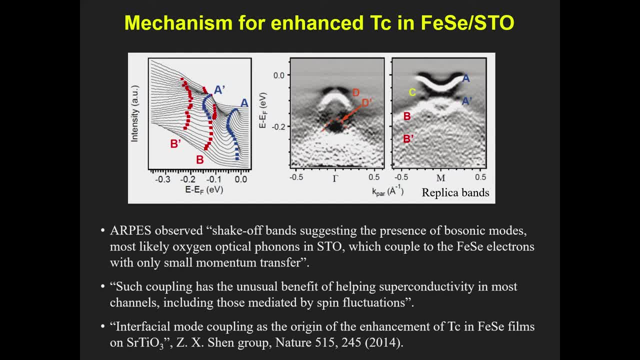 so, if I understand correctly, the spin fluctuations in ion selenide will give you an intrinsic Tc around 40 Kelvin. then from 40 Kelvin to 65 Kelvin, that's the enhancement due to the electrophonal coupling at the interface. so this is what we call. 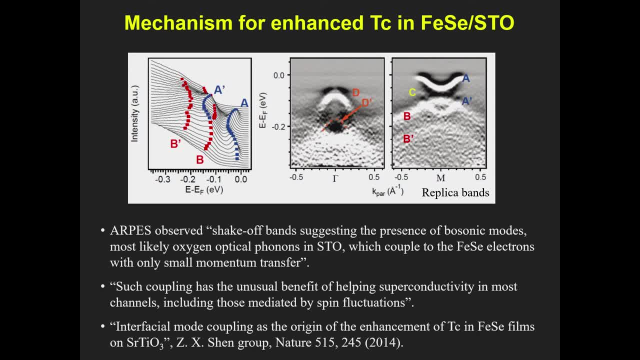 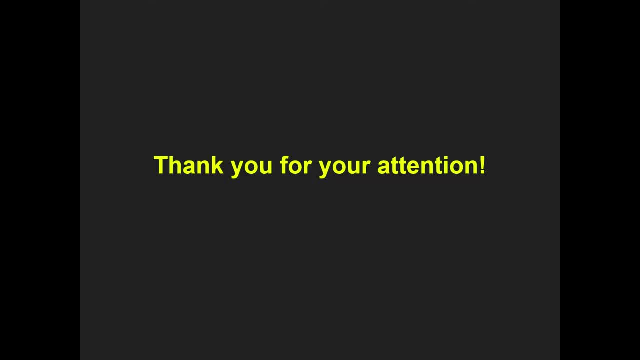 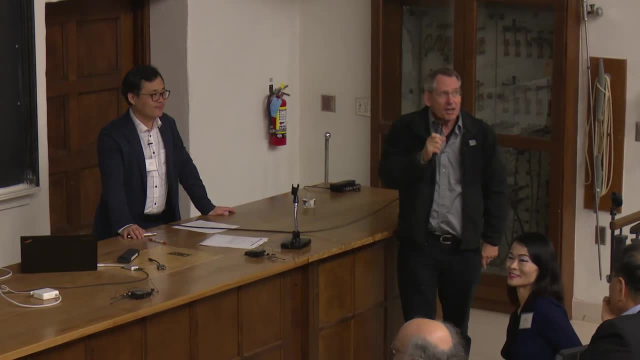 interface induced or interface enhanced high Tc superconductivity in this system. that's what I want to talk to you. thank you very much for your attention. alright, thanks for that fascinating talk. how are we doing on time? we are half an hour over. are we going to take? 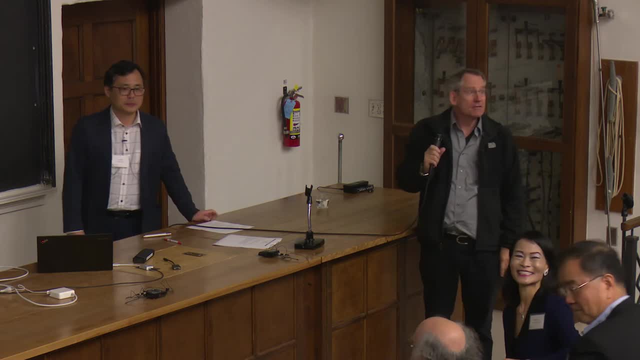 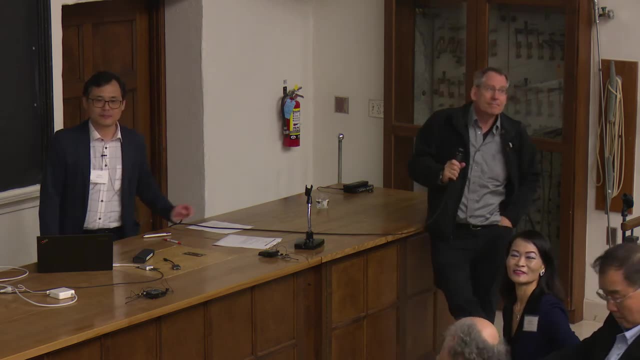 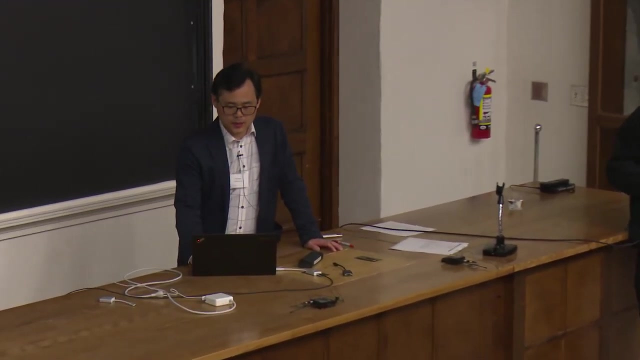 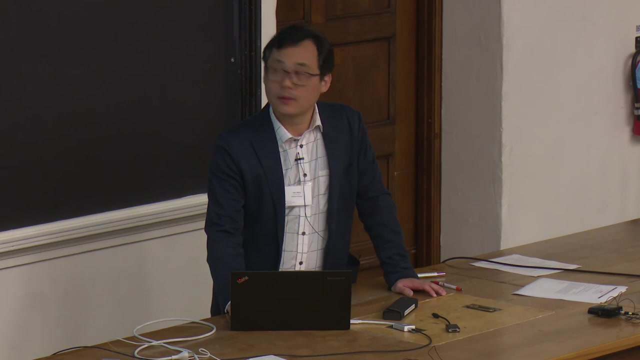 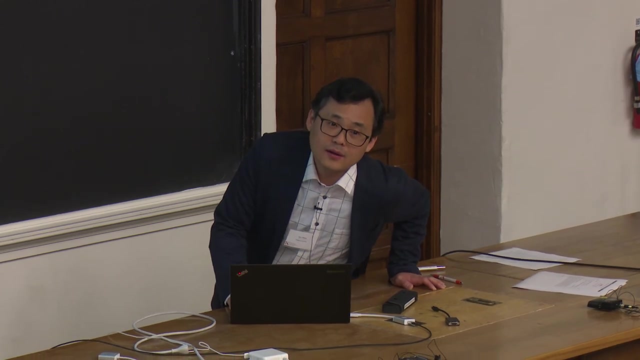 a question or two. we have time for a couple of questions. I noticed in your hysteresis loops, some of them in the quantum anomalous Hall effect. they were offset from zero. do you have an understanding of that? like what, like what before that, yeah, yeah. 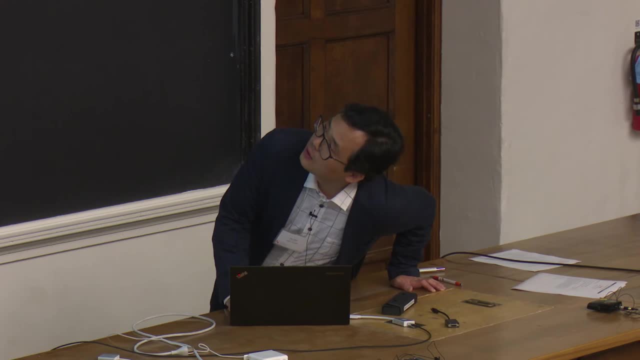 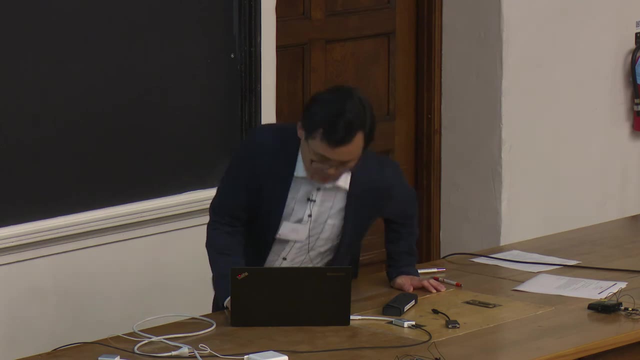 so why is it the switching field plus 0.1 and minus 0.2? wait, I think they are the same. it's around 0.1 and negative 0.1. here they are pretty similar. they almost match. if this was in a high field magnet. 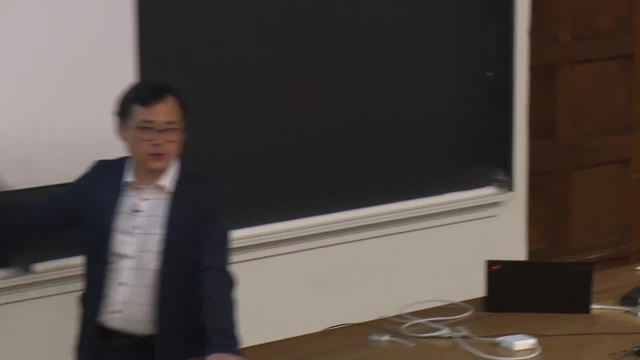 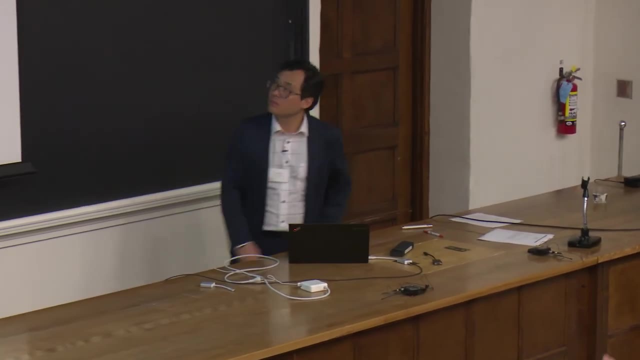 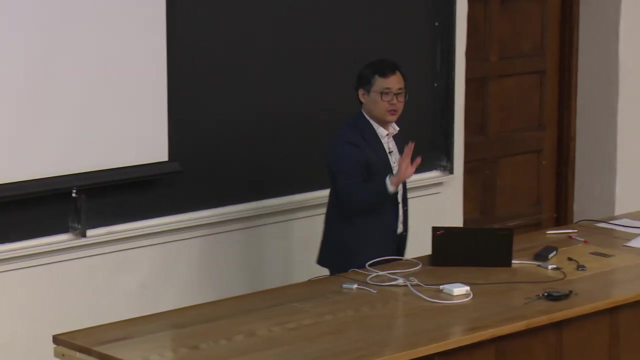 yeah, it's pretty, but I do see a little blip. that's right at 0, oh, at 0, that's different. I don't think it's. no, that's not due to the flux in the magnet, it's due to the rotation of the domains. 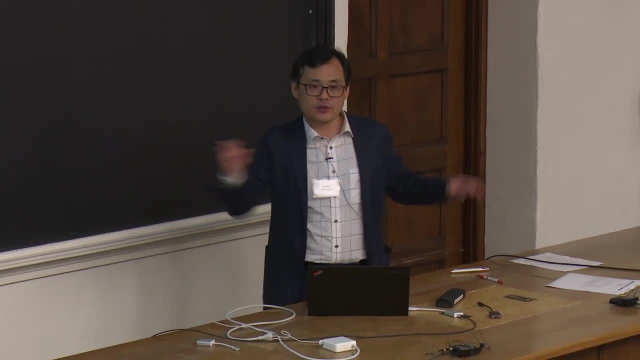 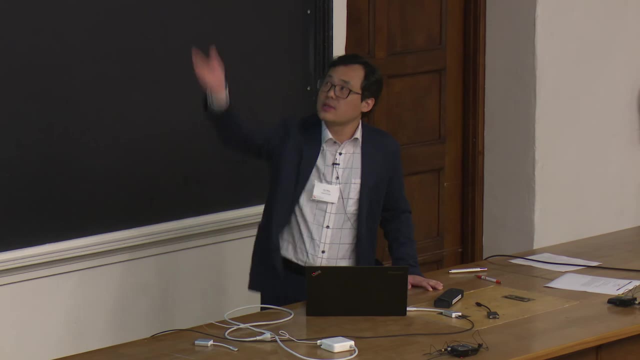 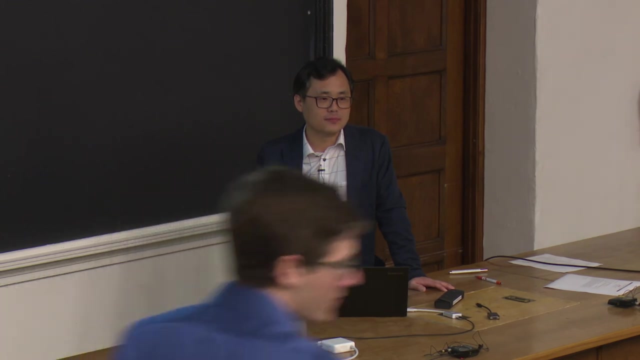 so as long as you reverse your magnetic field, the sample is highly homogeneous. there are some areas, small clusters with hysteresis, you know, because of the zero, so they will reverse first. so we see this in many materials, but not all of them. I have a question about. 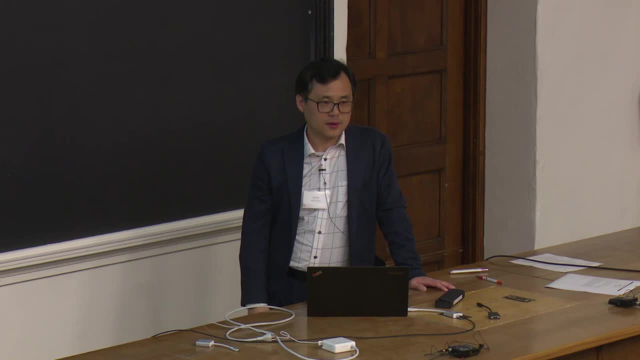 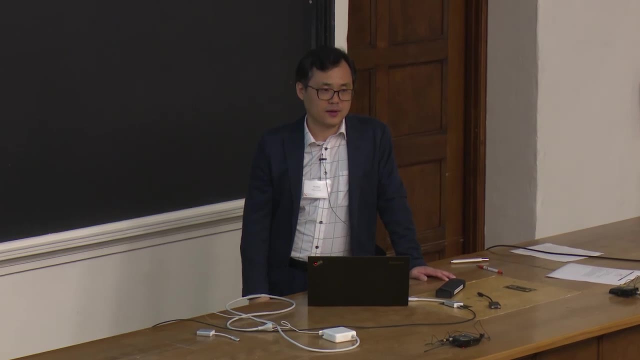 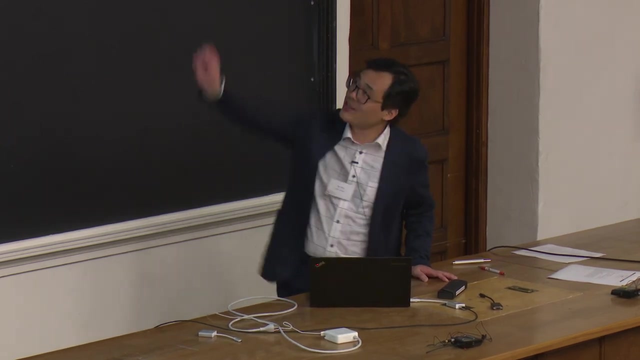 anomalous Hall. I noticed that at a zero magnetic field you suddenly have the Ixx. you see huge spikes, so suggest the system is like turning into insulator right, zero magnetic field. no, you shouldn't see that. no, it's not zero, that's a chorism field. 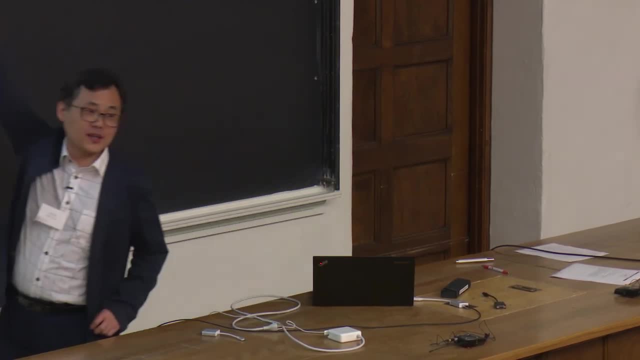 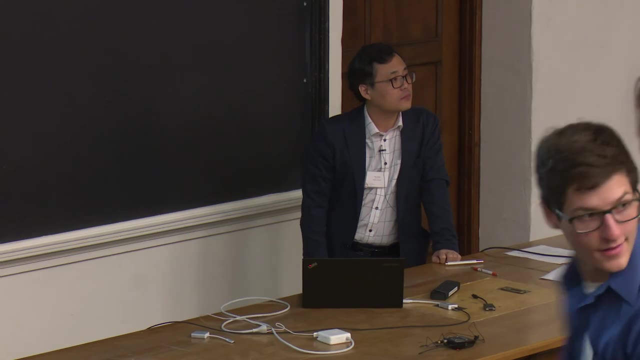 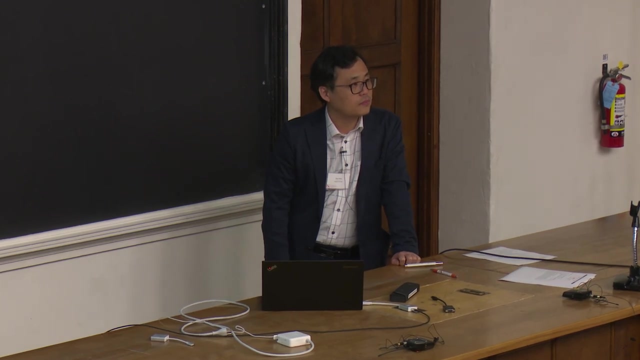 because the field scale is so large so you can see there are two peaks. that's when you again have the domain rotation scattering between them. a small comment: you have shown, like previous speakers, before, the skipping orbit picture in the integer quantum Hall effect. the group of in Stuttgart has looked. 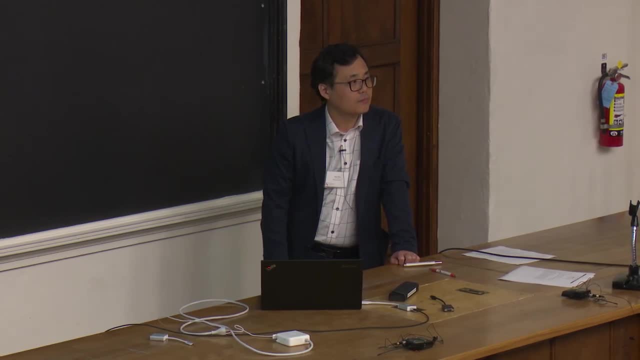 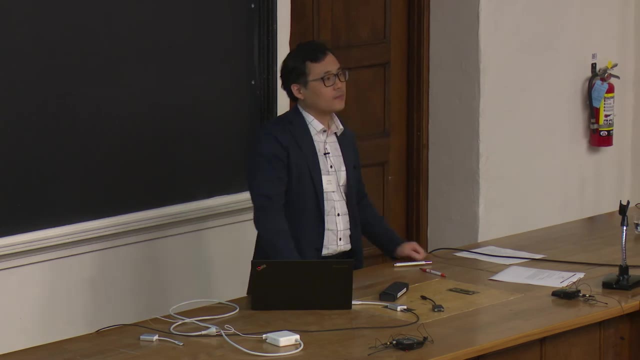 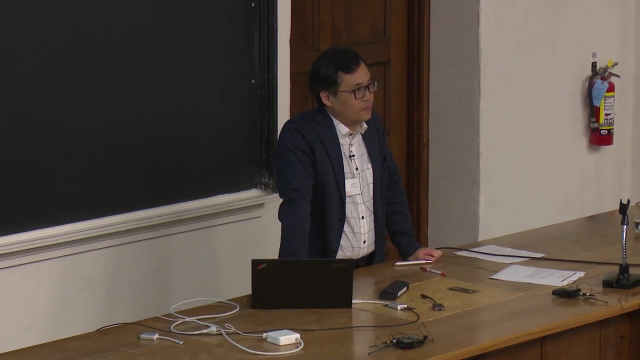 in detail where the current is flowing in the quantum Hall plateaus- doing, for example, scanning Hall probe, and they find that this skipping orbit picture does not apply at all. the current is either flowing in the bulk of the sample or in relatively broad stripes at the edges. 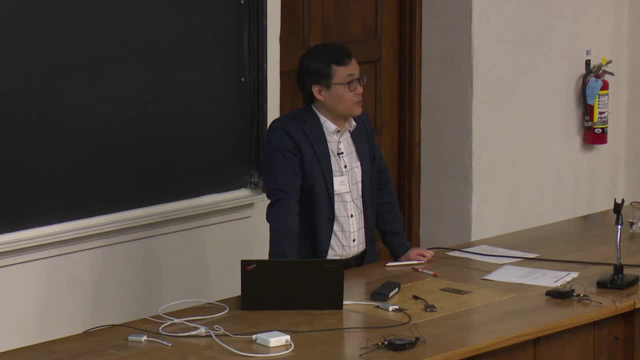 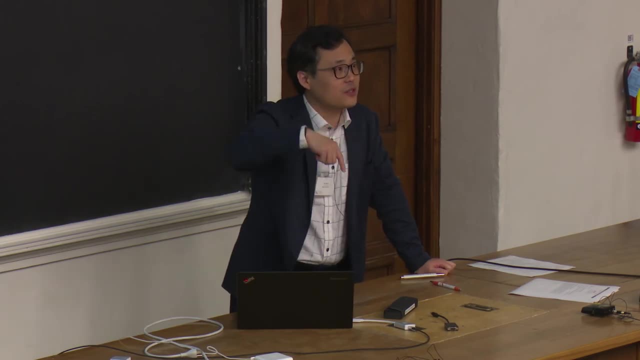 but not in a skipping orbit mode. yeah, yeah, that's a very good comment. I think there are some experiments, for example maybe in the group where they try to image the edge state, all the conducting channels in quantum Hall insulator. but the current flow has been imaged. 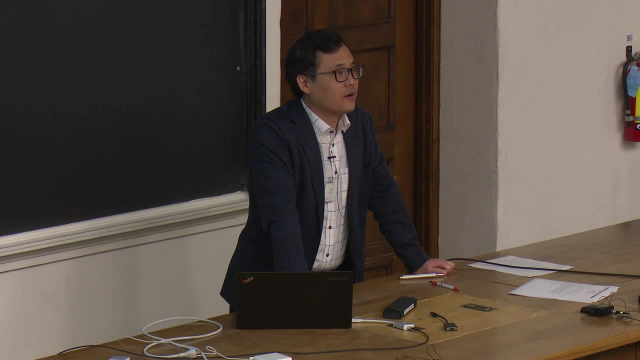 and this has been published and it's in the bulk or in broad edges, edge states. oh, you have the data already. yeah, it's out in quantum non-Hall insulator. no, in the standard integer quantum Hall effect. yeah, I'm talking about the quantum non-Hall insulator.